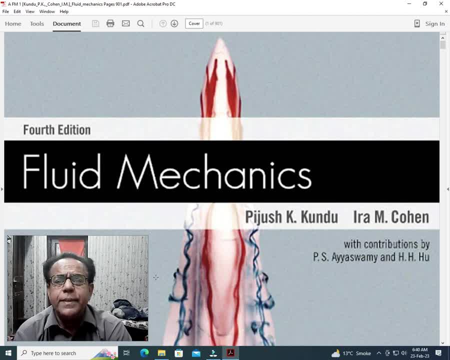 Fourth edition, fluid mechanics. P.J.K. Kundu, Ira M. Cohen, okay? With contributions by P.S. S. Vami and H.H. Hu. Dear students, again and again this thing is coming in front of me that author's names are very unusual. And I feel... 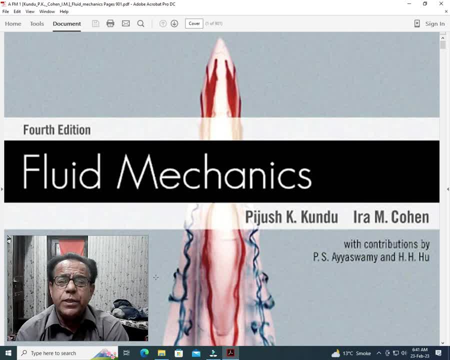 difficulty in pronouncing their exact names okay anyhow it is written in front of screen so even 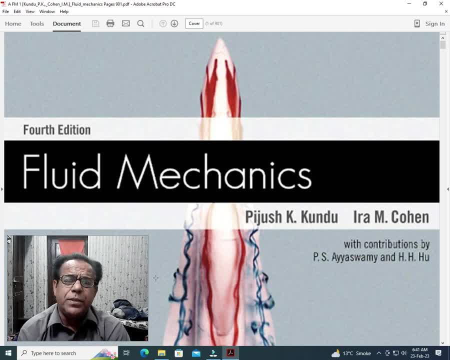 if I do not pronounce their names I think it will be okay but despite this I try to 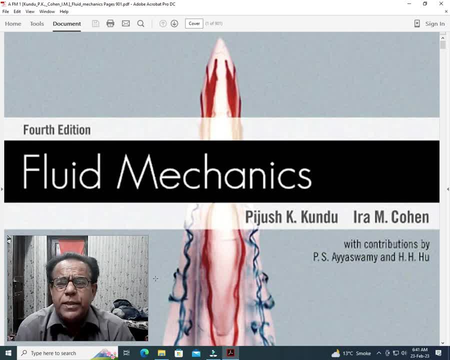 pronounce these names okay anyhow fluid mechanics fourth edition its authors are to look at the Jewish K kundu and Ira M Cohen with contributions by PSI a swami and HH you okay anyhow 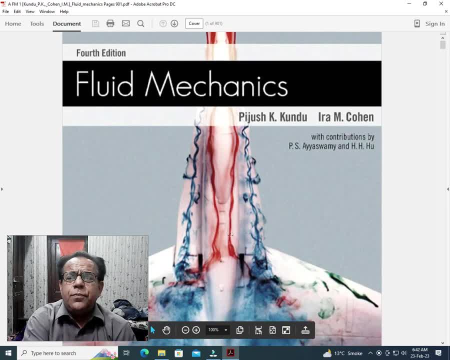 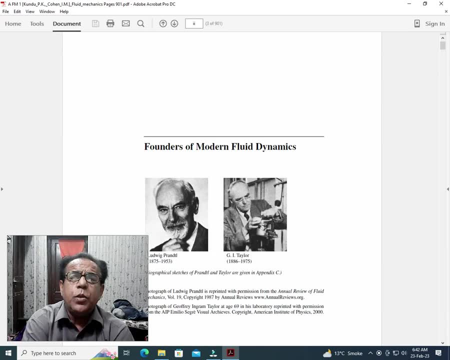 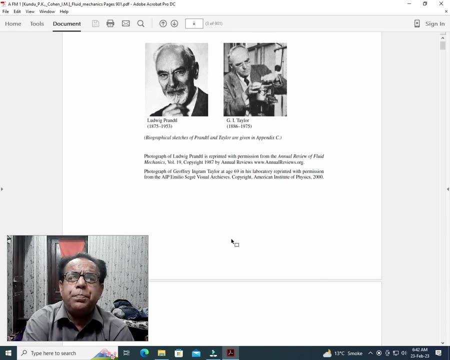 we move forward okay fluid mechanics fourth edition founders of modern fluid dynamics Ludwig Prandtl GI Taylor year of birth year of death year of birth year of death etc these are additional things 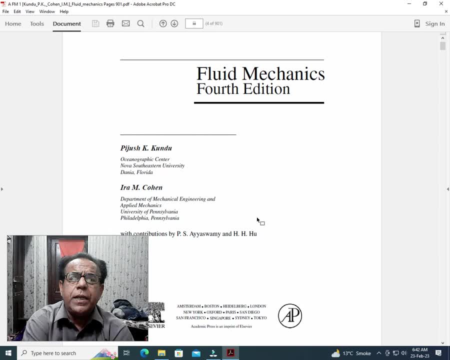 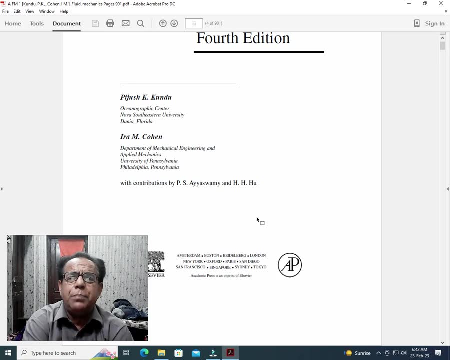 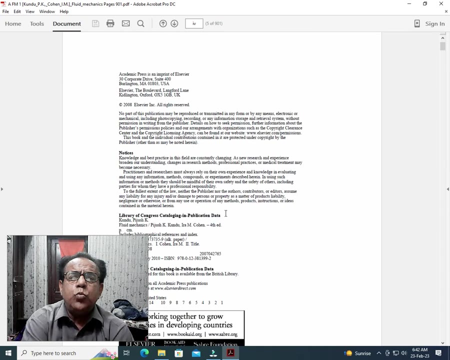 the fluid mechanics a bit Jewish K kundu Ira M Cohen with contributions by PSI a swami and HH you elsewhere is its publisher okay 2008 copyright 2008 yes because this is 4th edition 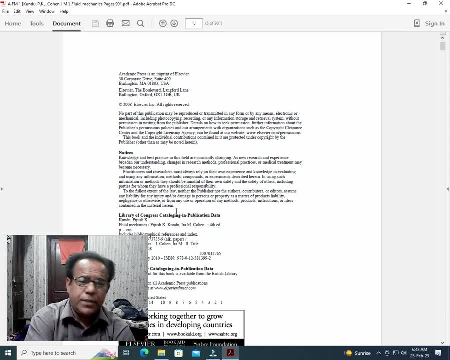 then there should be some information about the writer that this is the fourth edition then there should be some information about the writer that this is the fourth edition then there should be some information about the writer that this is the fourth edition information about previous three editions. But perhaps here that information does not appear and it will be perhaps it will be clear when we will go to prefaces then perhaps preface to first edition will be given then first preface to fourth edition will be given then preface to third edition then second then one and then 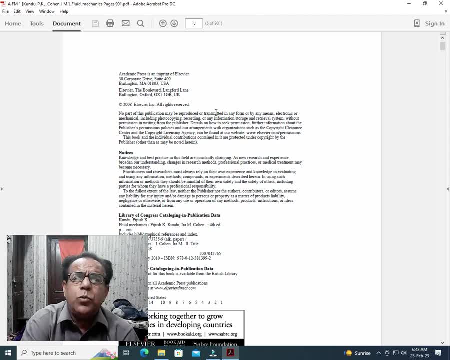 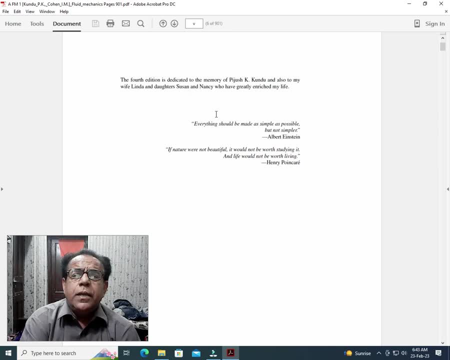 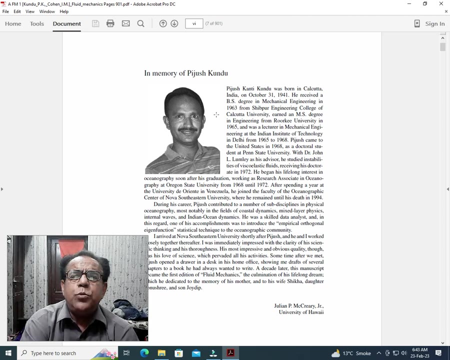 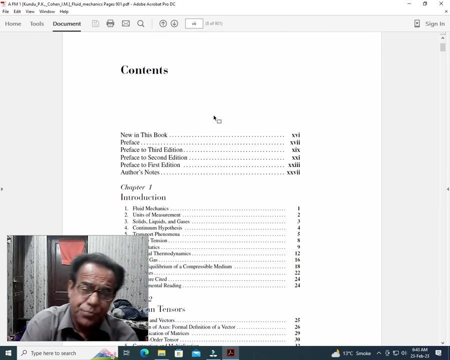 and from with the preface we will be able to know the years of publication of these four editions. Okay. Now we move forward. Okay. In memory of Piyush Kundu. Okay. Anyhow, first we come towards contents. Perhaps preface may be given after contents. While 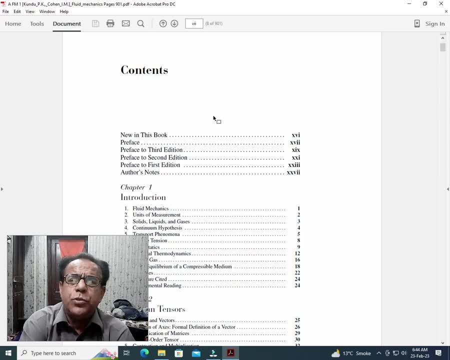 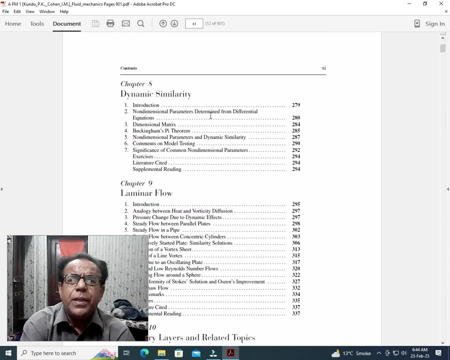 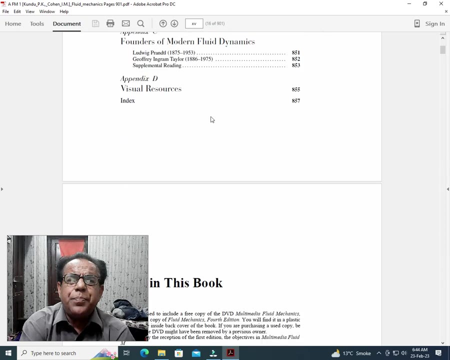 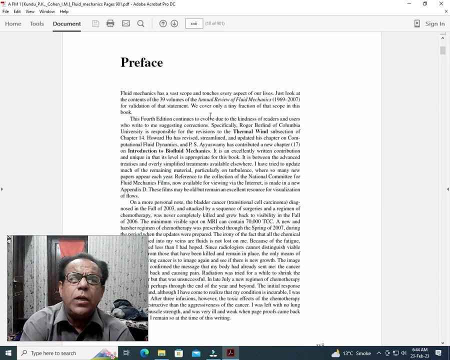 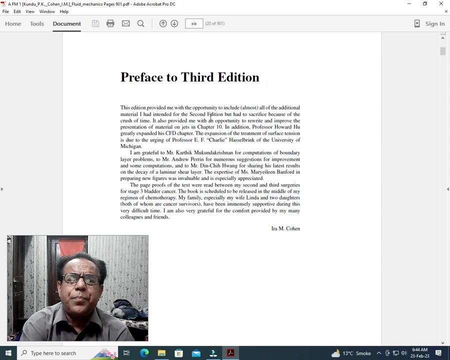 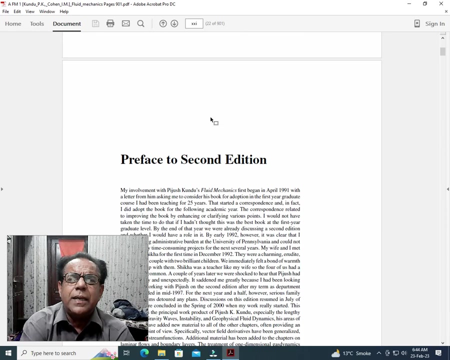 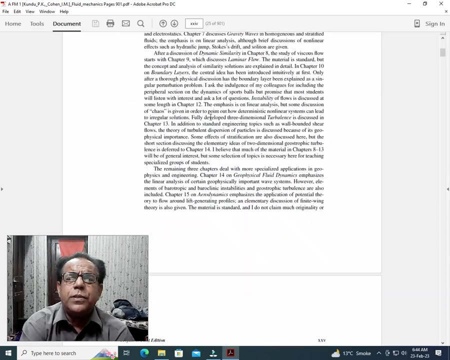 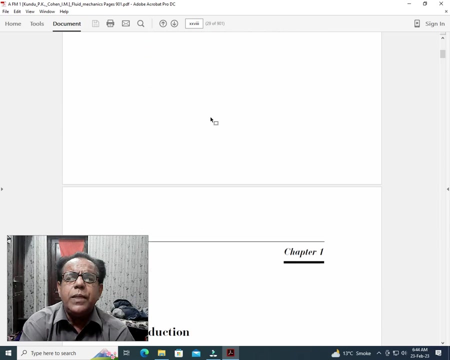 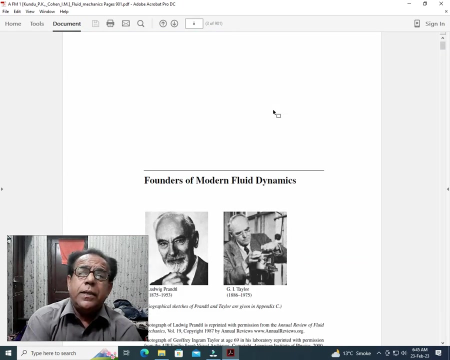 usual arrangement is contrary to this. Okay. Usually first preface is given and then contents appear. Okay. But in these soft versions of books having been downloaded from internet some irregularities may occur. Okay. So this is the preface situation. Yes. This is preface to third edition but year or date or month is not given. Okay. Preface to second edition here again not given. Preface to first edition here again date or month or year is not given. Okay. Anyhow, we now go back to its contents. Okay. 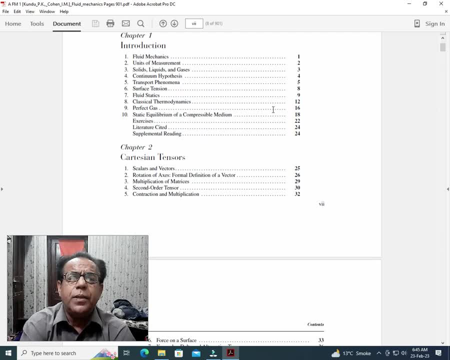 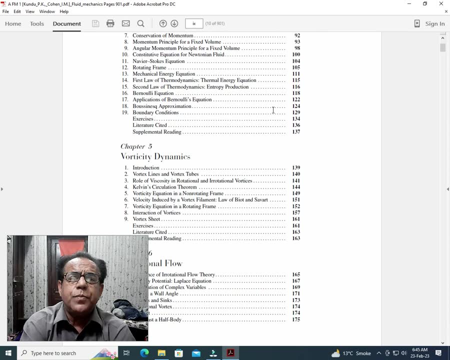 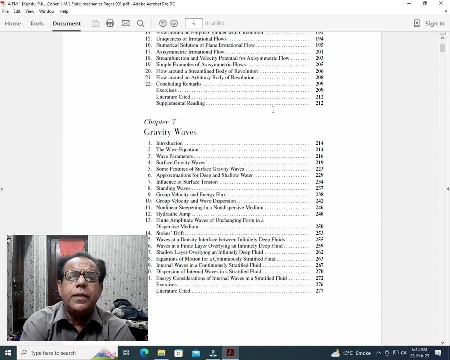 Yes. Contents. Okay. Introduction. Cartesian tensors. Kinematics. Conservation laws. Verticity dynamics. Irrotational flow. Gravity waves. Dynamic similarity. Laminar. 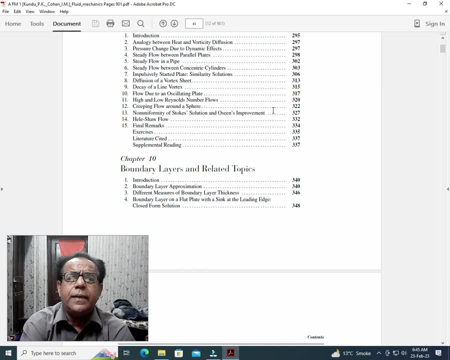 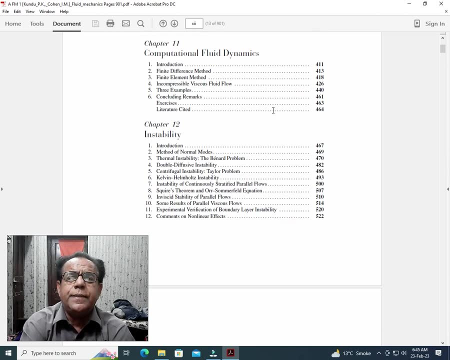 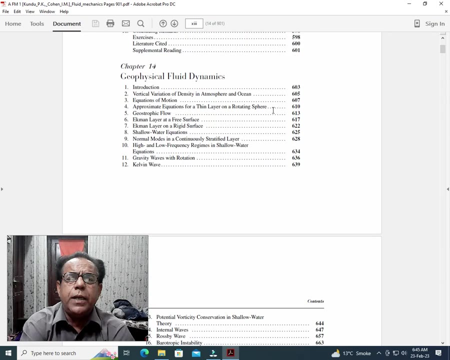 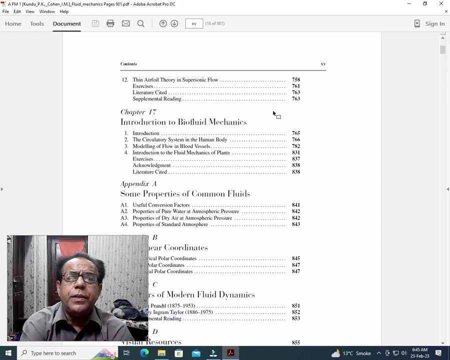 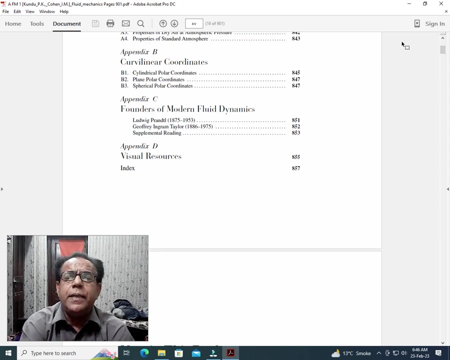 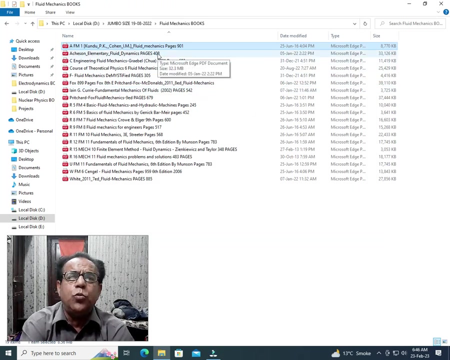 Car flow. Boundary layers and related topics. Computational fluid dynamics. Instability. Turbulence. Geophysical fluid dynamics. Aerodynamics. Compressible flow. Introduction to biofluid mechanics and then indexes. Indexes given at page number 857. Now we are going to open second book which consists of 408 pages. 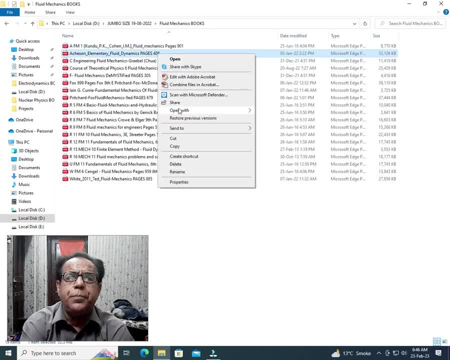 Okay. 408 pages book is being opened 408 pages. Okay. 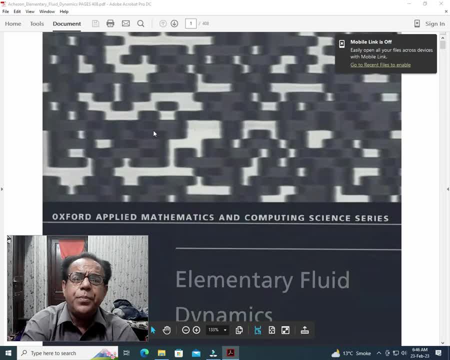 So dear students here is the situation. This book consists of 408 pages in accordance with soft. 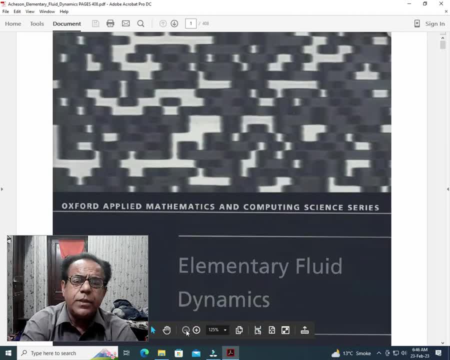 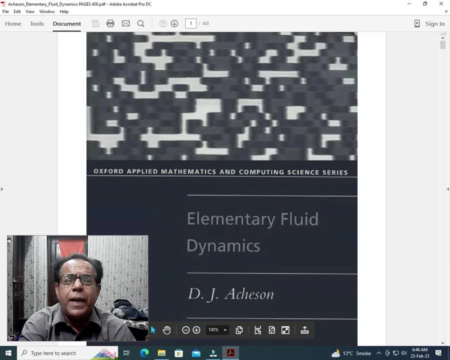 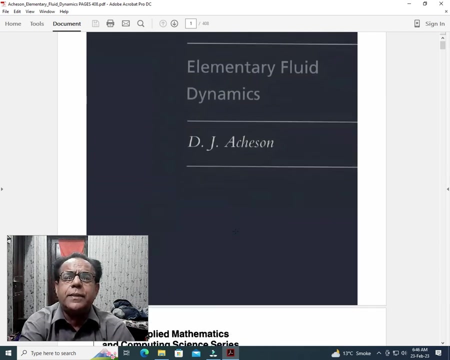 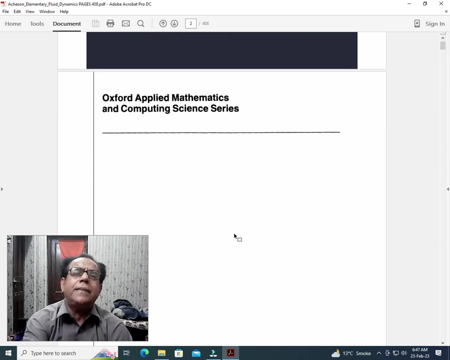 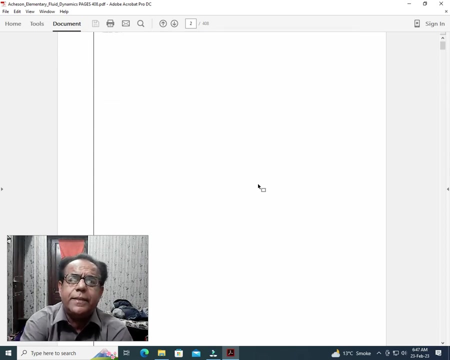 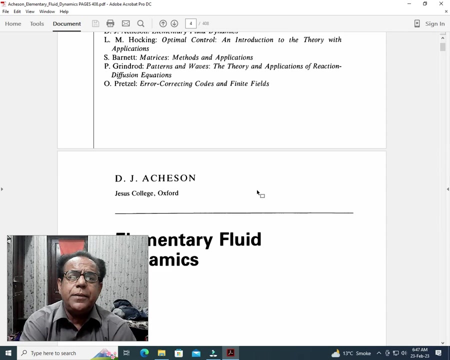 soft copy arrangement okay oxford applied mathematics and computing science series okay oxford applied mathematics and computing science series elementary fluid dynamics DJ a chisholm DJ a chisholm DJ a chisholm okay oxford applied mathematics and computing science series oxford applied mathematics and computing science series DJ a chisholm elementary fluid 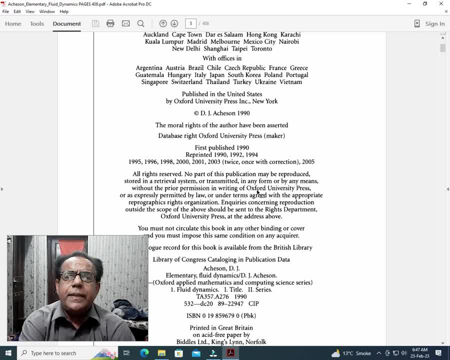 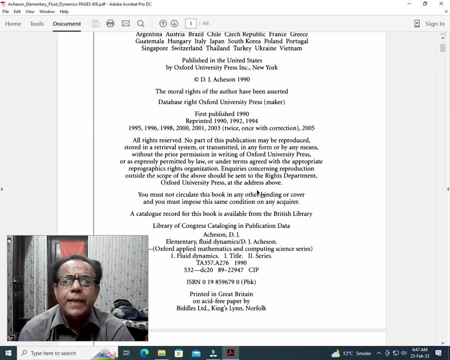 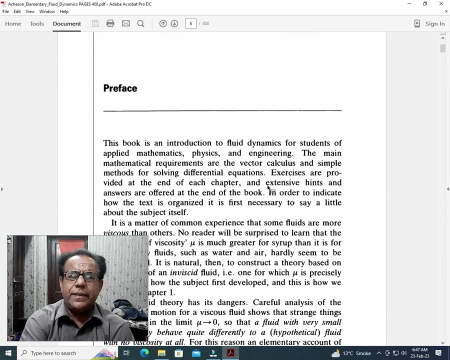 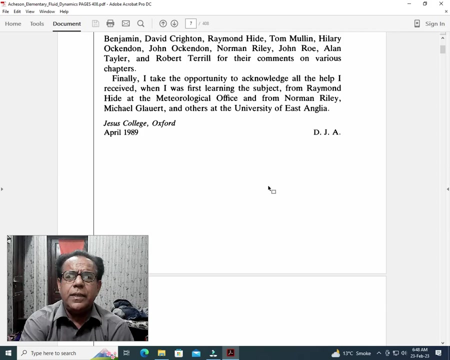 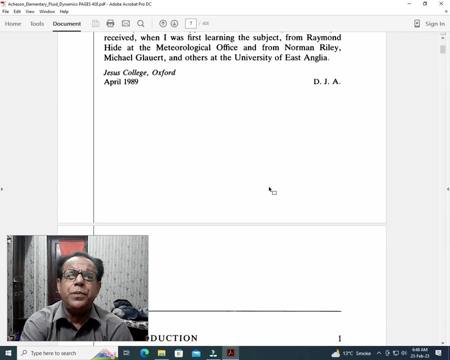 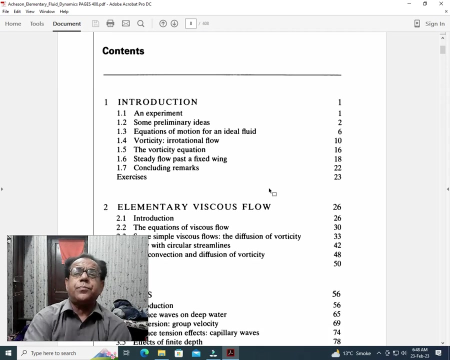 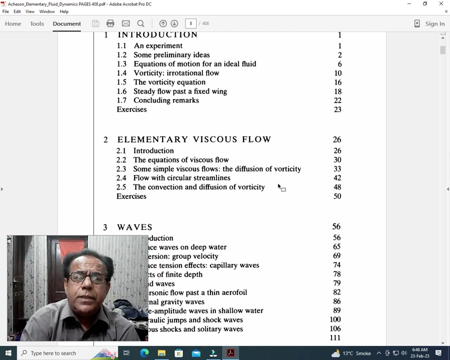 1990 copyright okay however previous years are also given okay first published in 1990 then reprinted in 1990 92 94 95 6 8 2000 2001 2003 okay anyhow these are unnecessary less relevant things it's a preface was written in April 1989 okay whether it is yes it is preface sometimes in place of preface a word forward is used that is also a similar thing okay anyhow we come towards the contents okay first chapter is the introduction second elementary viscous flow waves classical aerofoil 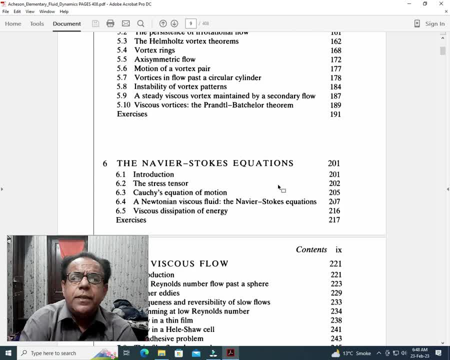 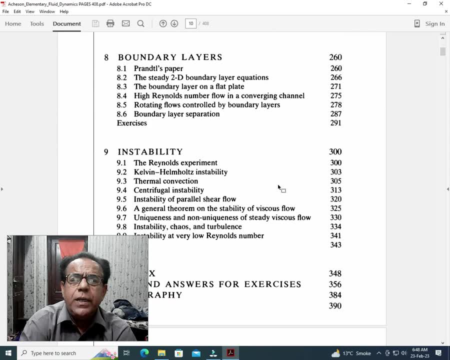 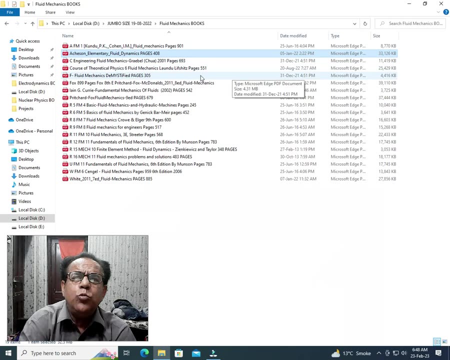 vortex motion the navier-stokes equations very viscous flow boundary layers instability and index is given at page number 390 okay now we can move to next book which consists of 693 pages and this is addition of year 2001 engineering fluid mechanics 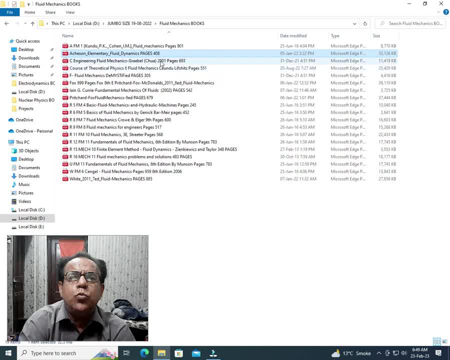 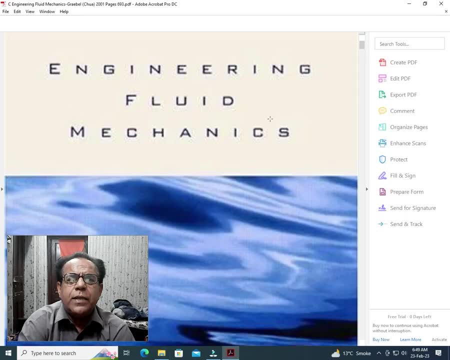 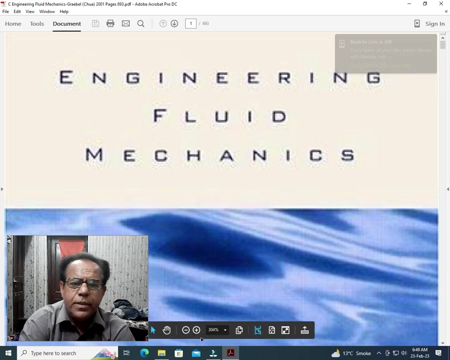 now in this book we will be seeing a example of what is the name of sp WEA you 5 20 20 20 200 200 250 300 300 330 350 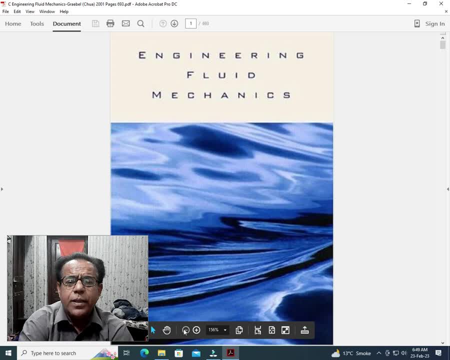 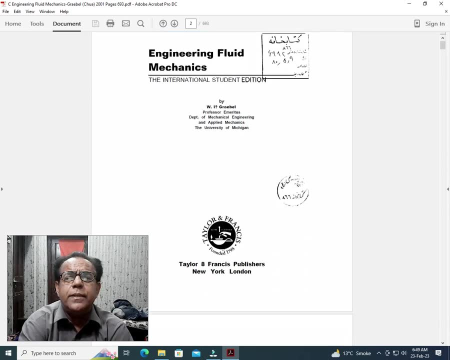 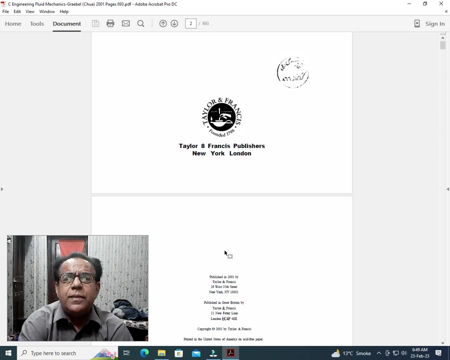 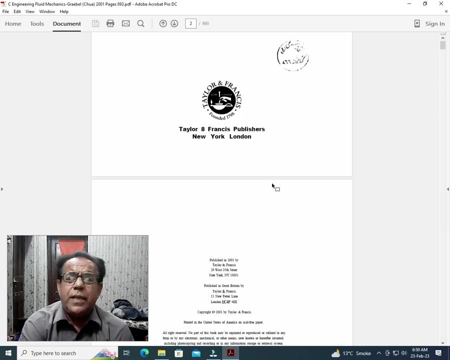 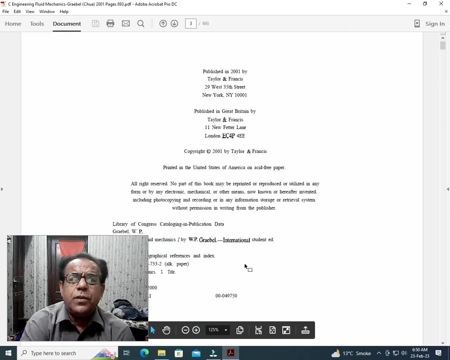 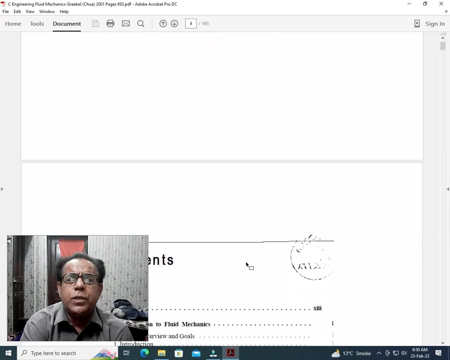 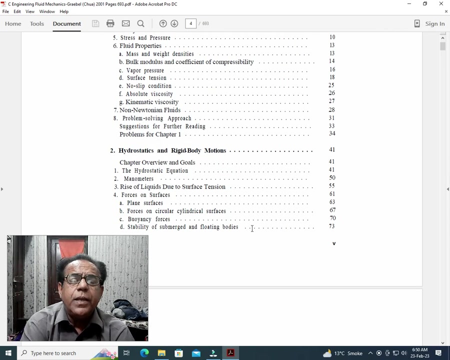 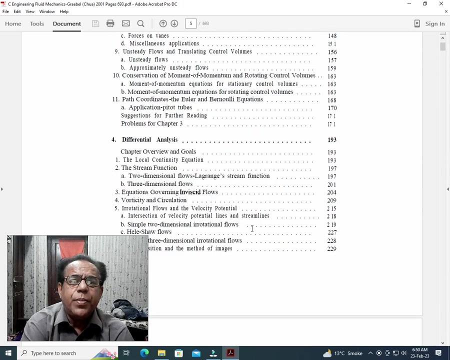 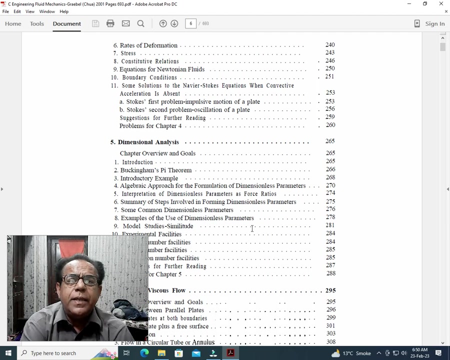 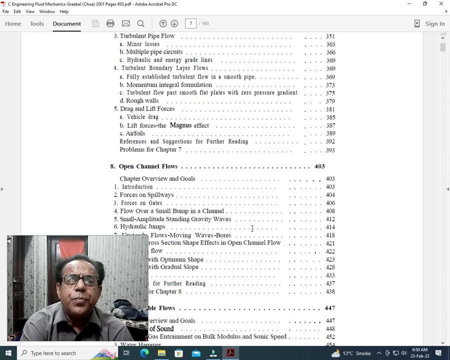 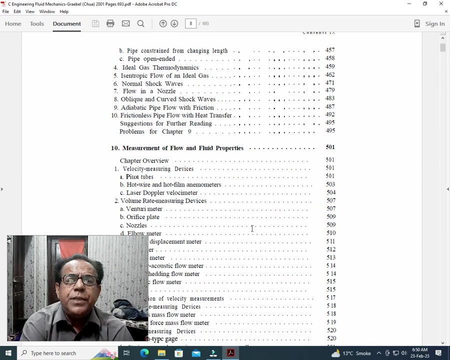 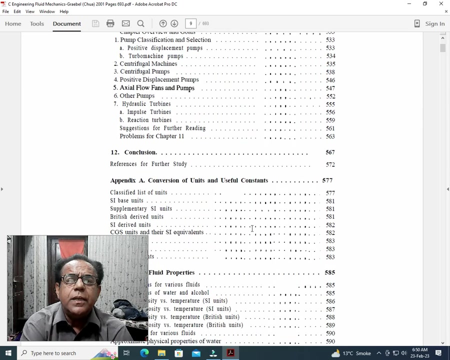 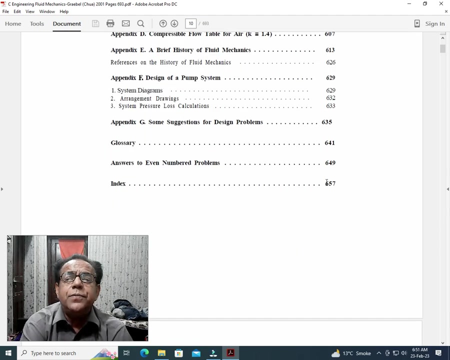 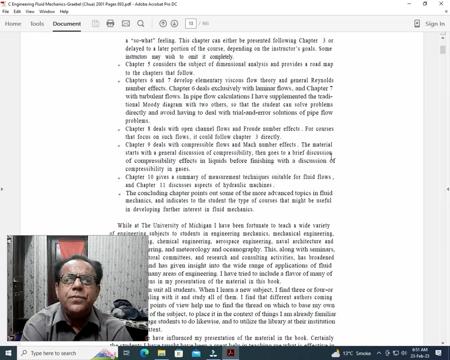 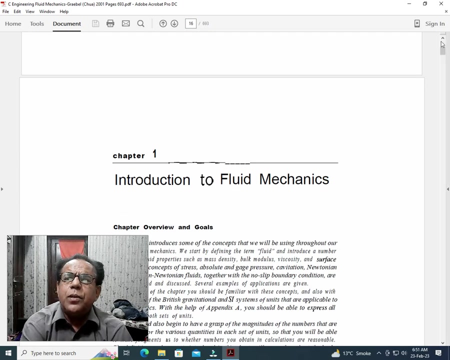 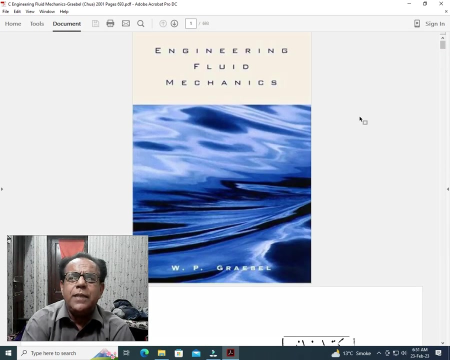 240 Engineering Fluid Mechanics. Okay. Engineering Fluid Mechanics. The International Student Edition. Taylor and Frankis Publishers. Okay. Here students you can see that Taylor ate Frankis Publishers. Okay. Actually this is Taylor and Frankis but mistakes always occur. Okay. Anyhow. Anyhow. Anyhow. 2001. Okay. This book was published in the year 2001 by Taylor and Frankis. Okay. Now we come towards its contents. Okay. Introduction to Fluid Mechanics. Hydrostatics Add Rigid Body Motion. Okay. Fluid Dynamics. Differential Analysis. Dimensional Analysis. Laminar Viscous Flow. Turbulent Viscous Flow. Open Channel Flows. Compressible Flows. Measurement of Flow and Flow Proximity. Properties. Hydraulic Machinery. Conclusion and Index is given at page number 657 of this book. Okay. And now we can safely. Yes. We see preface. Okay. No year at given. Yes. Now we can safely move to. But here this one thing has remained doubtful that why I had used the word chua and I said that chua is we say chua to rat in our local language. There might be something like CHU. CHUA. Okay. Okay. Okay. Okay. Okay. Okay. Let us once again. Okay. Okay. Okay. Okay. Okay. Okay. Okay. 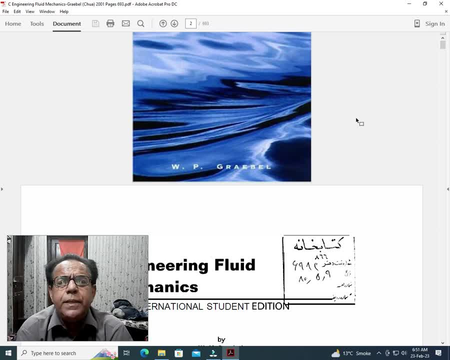 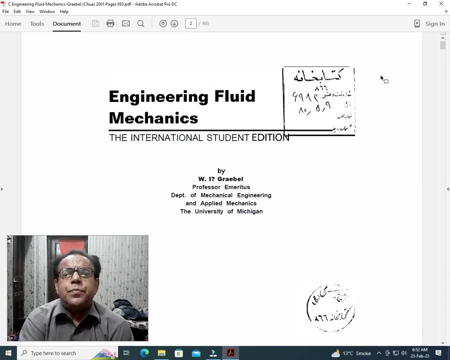 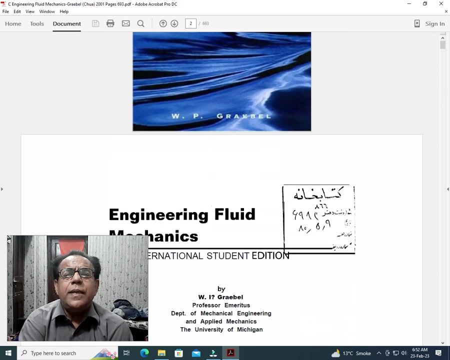 It's author is W. P. Grable. Okay. It's author is W. P. Grable. G. R. A. E. B. E. L. W. P. Grable. Okay. Here once again mistake seems. Here it is written W. P. Grable. But here W. 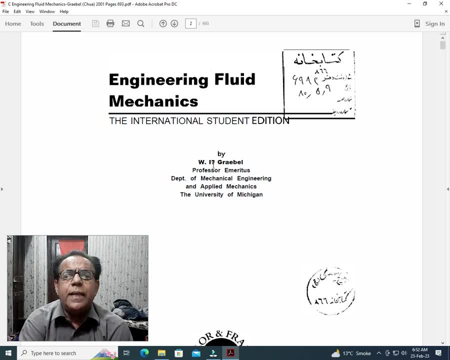 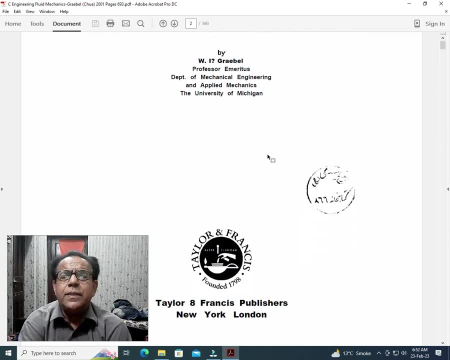 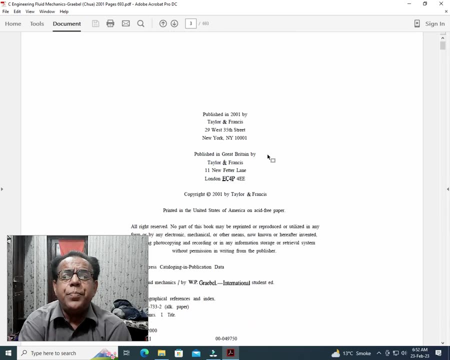 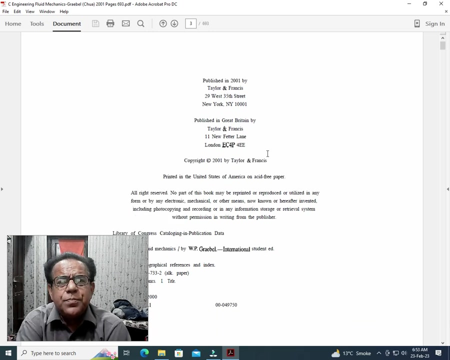 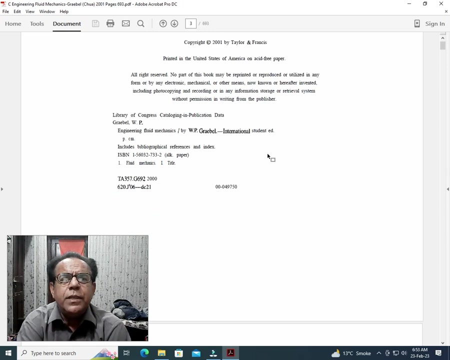 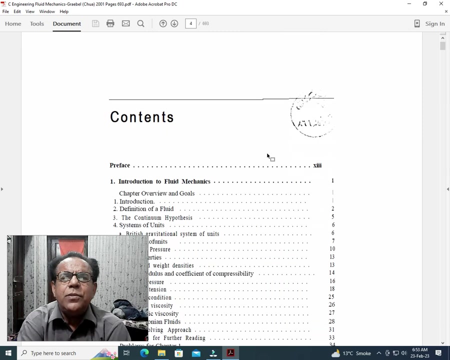 dot I then then sign of integration grapple okay this is a mistake Taylor and Frank is now we try to find out that at the time of saving this book in my computer I used within bracket CHU a CHU a I do not know why I why did I use this word while saving this book in my computer okay we take some time and then we will assume you 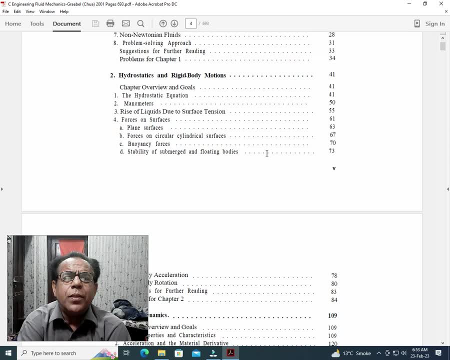 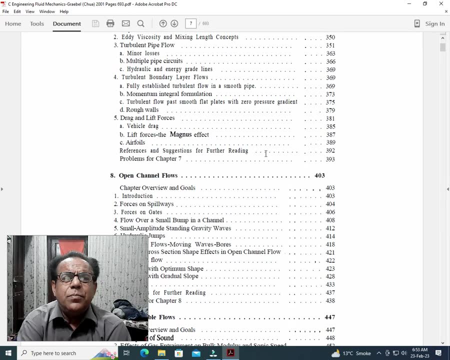 that it was by mistake okay perhaps it needed to be written China any how 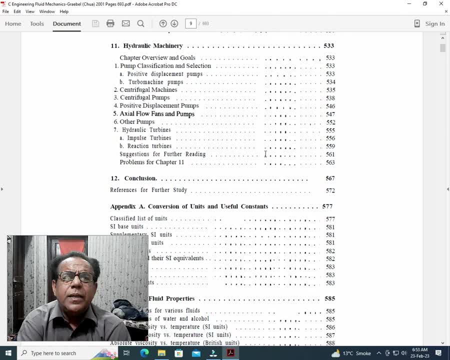 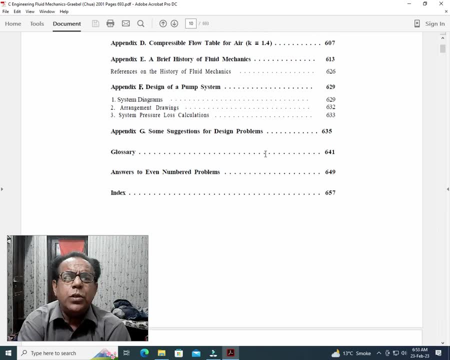 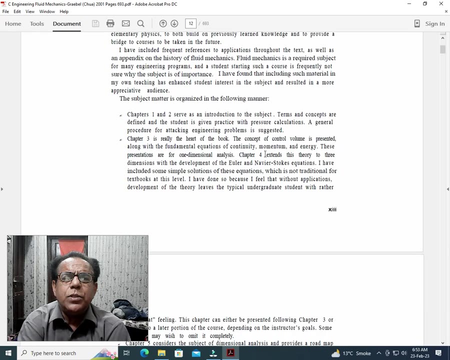 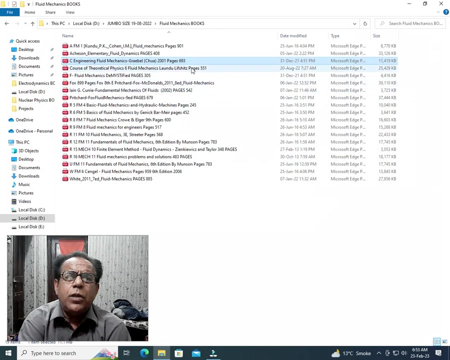 actually dear students several years have gone in such books having been saved in my computer so I do not know why I did use word CHU a while saving this book in my computer 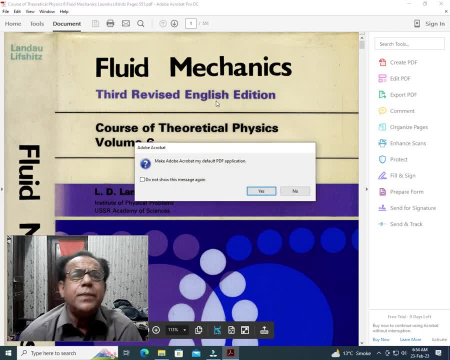 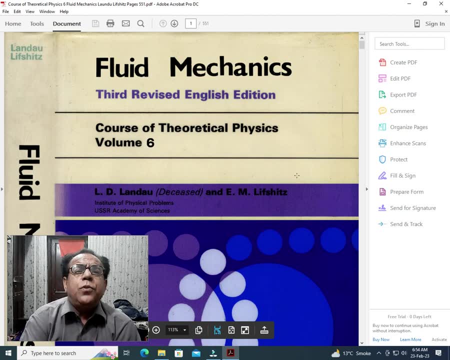 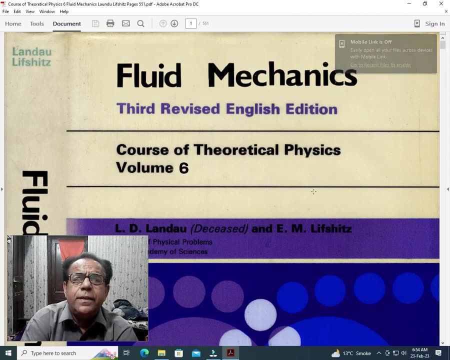 okay next book next book consists of 551 pages okay flu lando live sheets okay lando live shit sir this is clearly based on the English version of this instruction and we have to just get rid of her photos too sorry okay this was the one I was reading earlier all right go aheadOUT 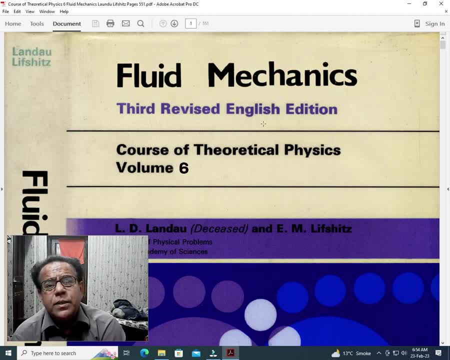 HR this is the first chapter okay 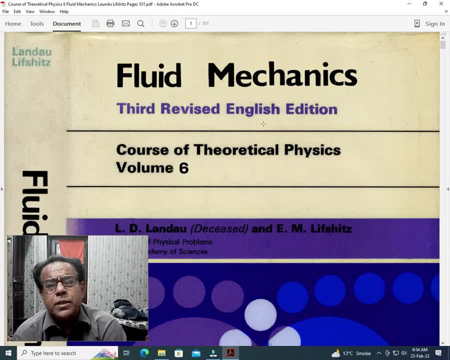 please simple color and I did not read all well 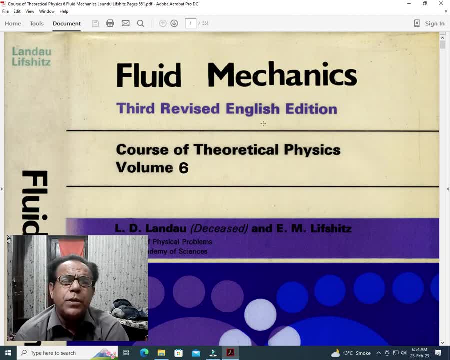 and not make anyitatio use that lines Charlin done the point work should be in print curly hair anyhow okay framing textiles at loved것 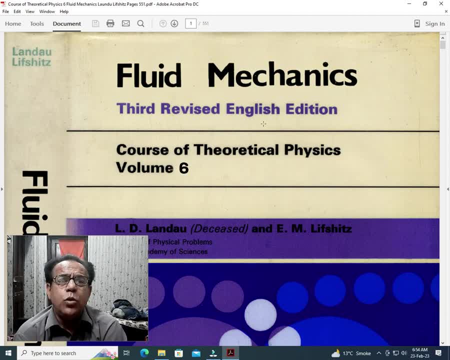 of theoretical physics volume 6 by landu leaf sheets okay dear students here we should make 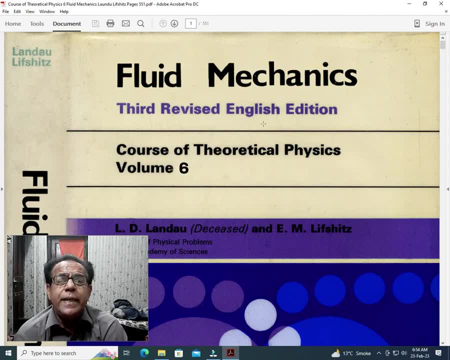 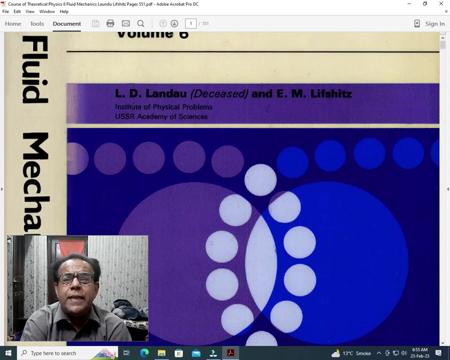 it clear that this volume 6 indicates that this authors has several other books under the same name course of theoretical physics okay but the only difference is that here volume 6 is regarding fluid mechanics it is quite possible that volume 5 may relate to classical mechanics volume 2 may relate to quantum mechanics and so on okay ld ladu deceased and em leaf sheets okay institute of physical problems 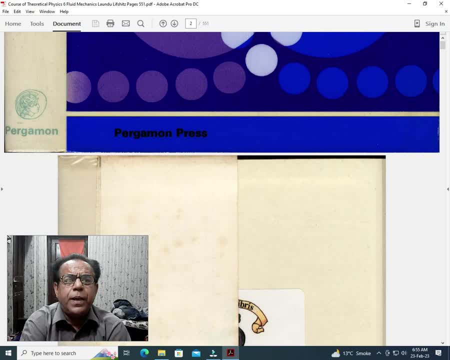 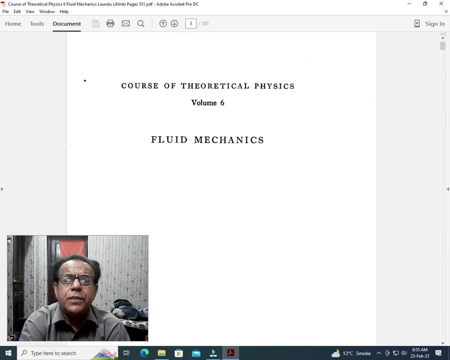 anyhow we go forward pergamon pergamon is the publisher of this book okay course of theoretical physics volume 6 fluid mechanics oh yes what i said 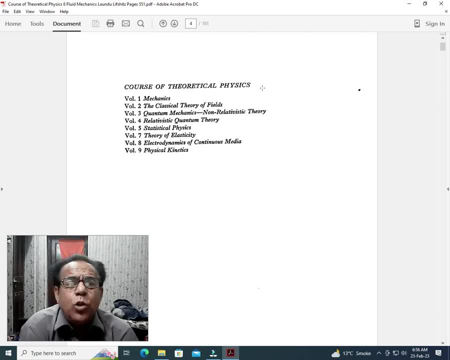 has now become quite clear that this volume 6 here you can see that volume 1 2 3 4 5 7 8 9 oh okay so at this point you can see that volume 6 has been omitted from this list because currently we are dealing with volume six by remaining eight volumes okay volume one is simply general mechanics volume 2 is about classical theory of fields volume 3 is about quantum mechanics non-relative relativistic theory volume 4 is about relativistic quantum theory volume 5 is about statistical physics with relativistic quantum theory volume 7 is about present quantum economics volume 6 is about volume 7 is about theory of elasticity volume 8 is about electrodynamics and continuous media and volume 9 is physical kinetics okay so dear students if we feel this book helpful and written 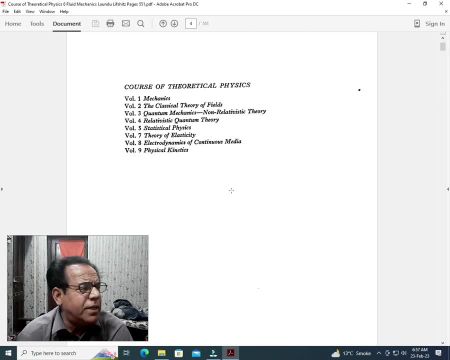 in an easy manner and we declare this book as our favorite then definitely we should go to these remaining eight volumes by the same author okay but if we we are not satisfied with this volume that is volume six year then I think we should not try to warnings 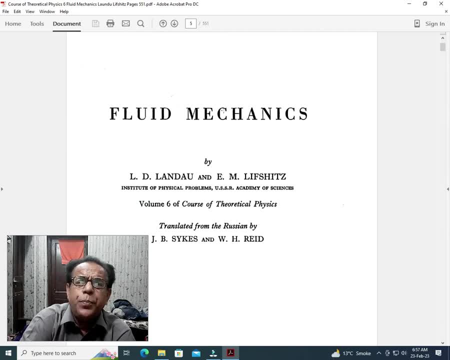 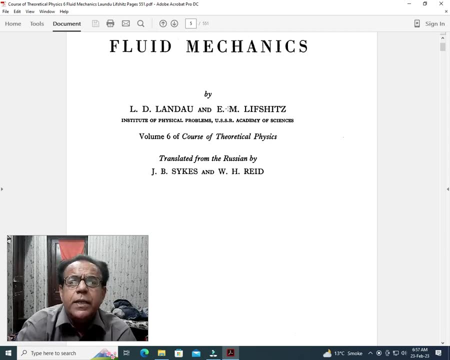 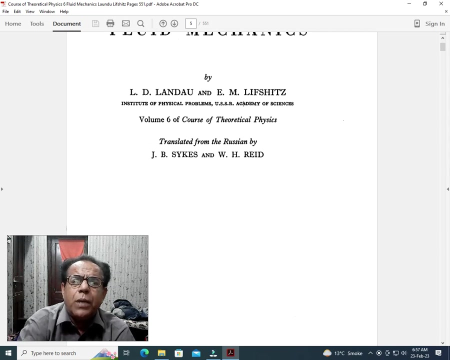 books by L.D. Landau and E.M. Lipschitz volume 6 of course translated from the Russian by J.B. Sykes and W.H. Reid read or write okay so these two persons had translated this book from Russian language okay the Pergamon Press is the 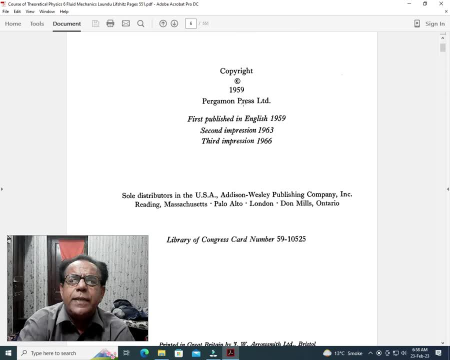 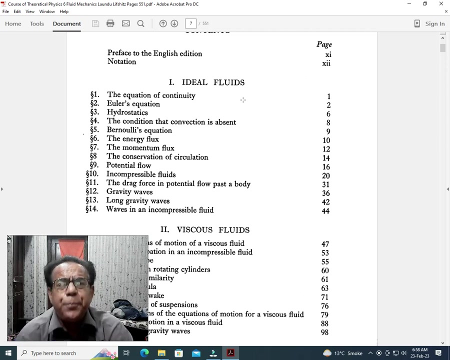 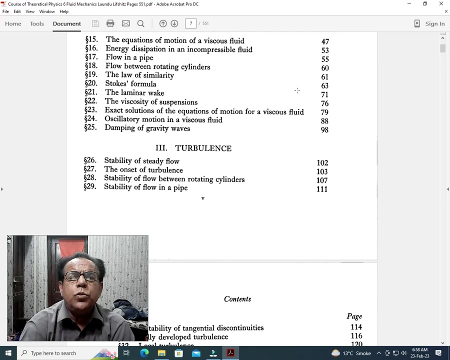 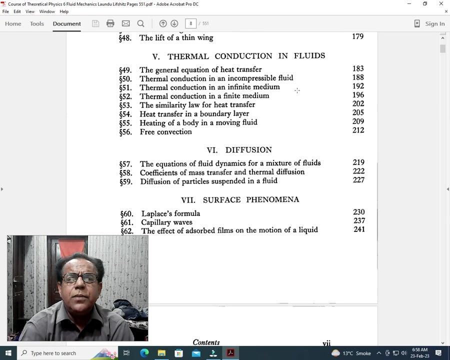 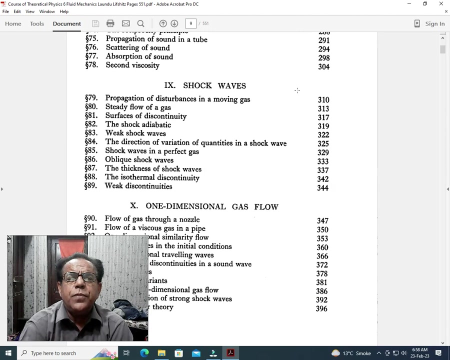 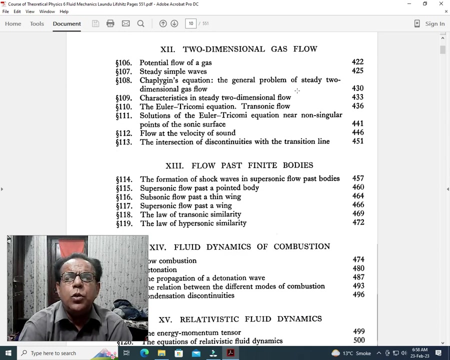 publisher of this book and copywriter of 1959 then a second impression in 1963 1966 okay so dear students a very old book 1959 okay ten years prior to my year of birth okay anyhow we come towards its contents okay ideal flutes Viscous Flutes Turbulence Boundary Layers Thermal Conduction in Flutes diffusion surface phenomena sound shock waves one-dimensional gas flow two dimensional gas flow flow past finite body flow fluid dynamics of combustion relativistic flutes 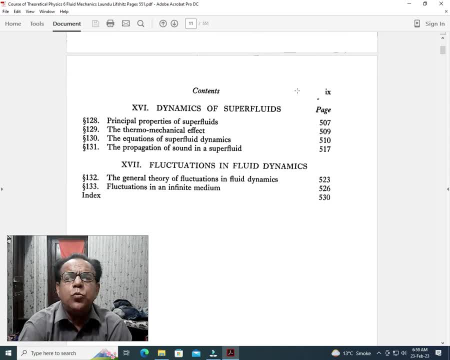 dynamics dynamics of superfluids fluctuations in fluid dynamics and then the preface 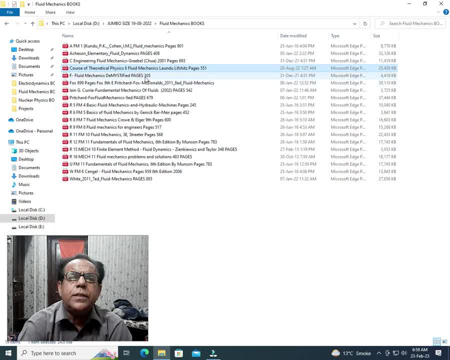 okay now we can move to next book which consists of 305 pages okay 305 pages book is being opened 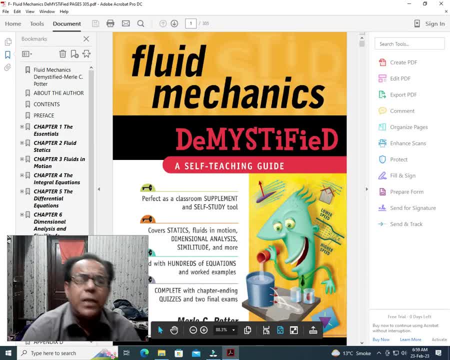 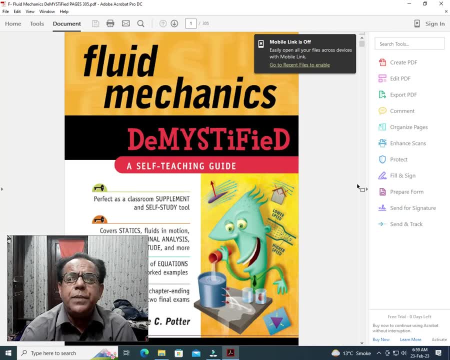 yes this is the book of 305 pages 305 pages in soft format okay soft format means that this numbering does not 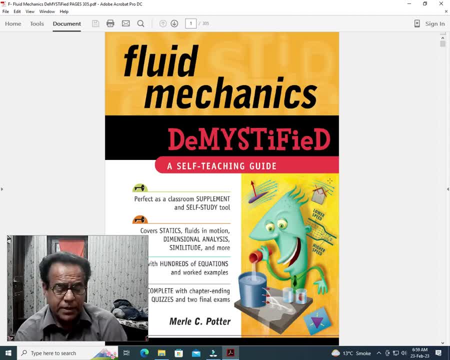 tally or correspond exactly with the number of pages 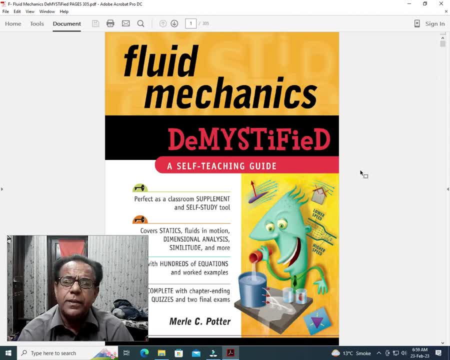 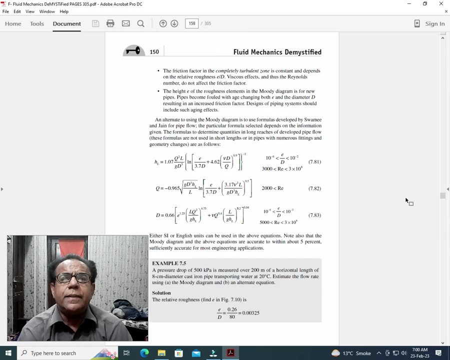 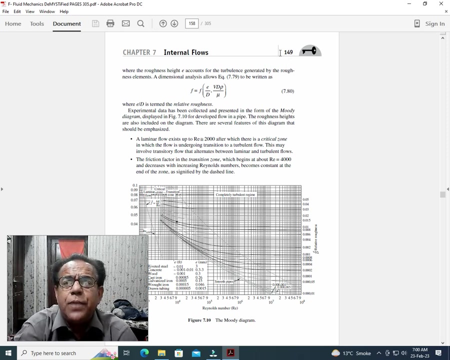 printed in hard format at papers of this book so for example i i dear students say i show here okay yes for example yes dear students you can see here this is page number 149 okay which is printed on papers of this book when we will take print of this book our hard copy will say that this is page number 149 okay 149 will be printed in the hard copy of this book here but here as per soft copy arrangement this is page number Okay, so nine pages difference. Why nine pages difference? Nine pages difference is that if we start this book, then first nine pages will be extra additional pages and regular first page will start from page number 10. 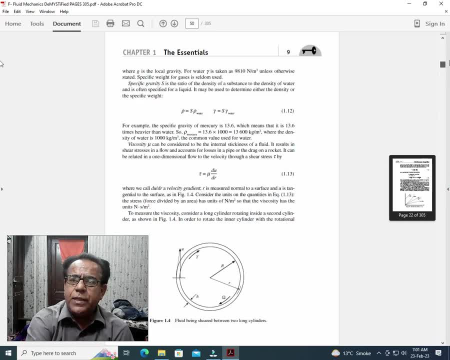 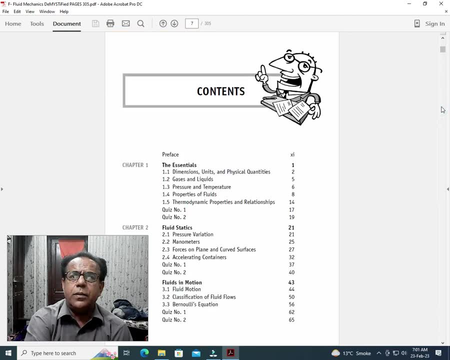 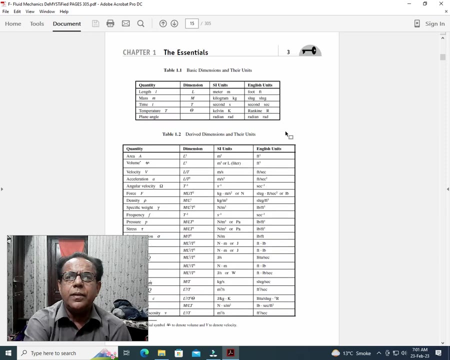 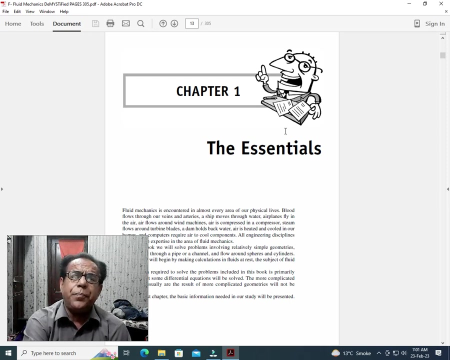 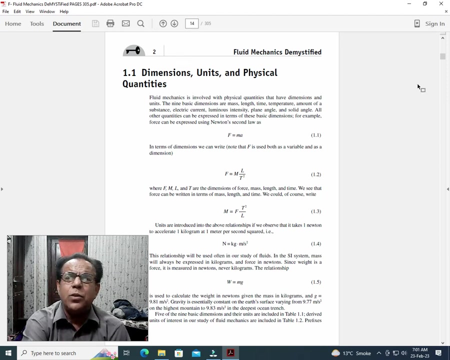 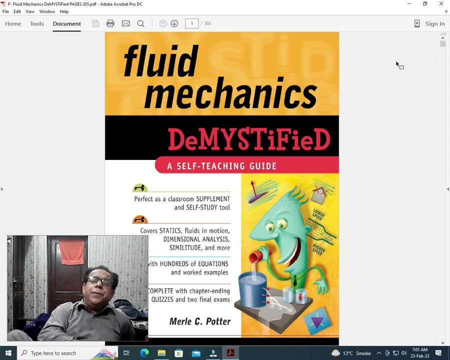 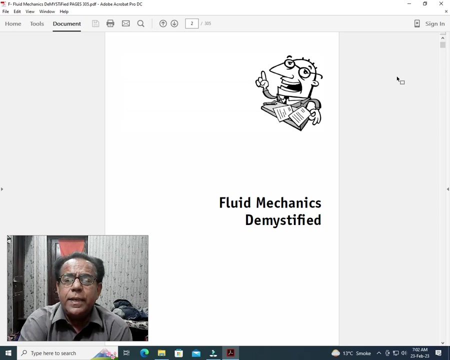 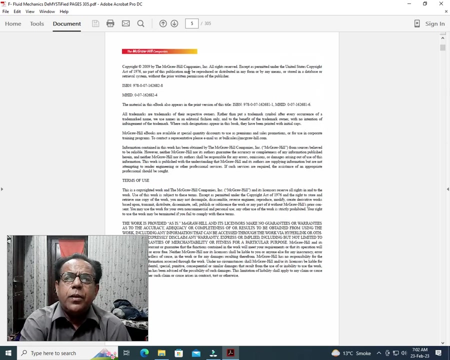 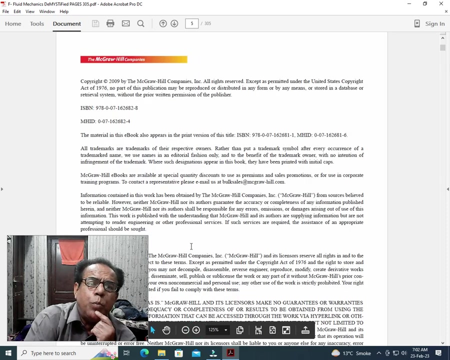 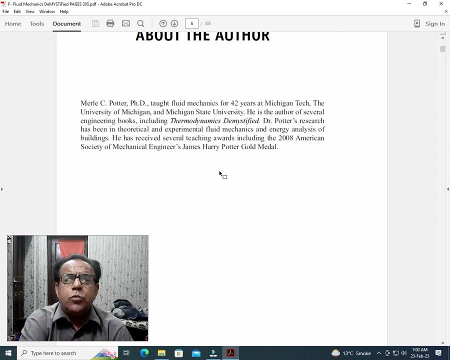 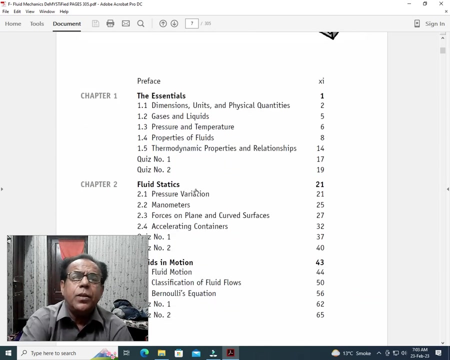 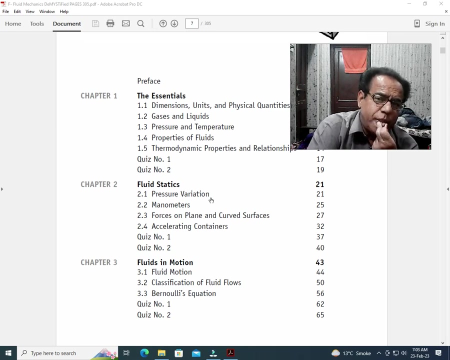 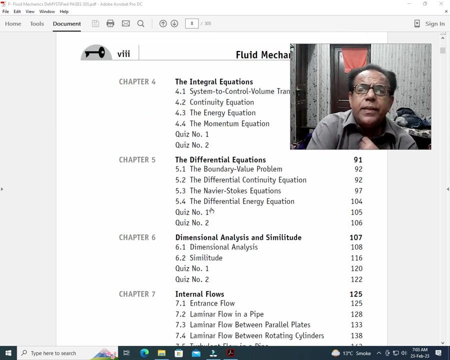 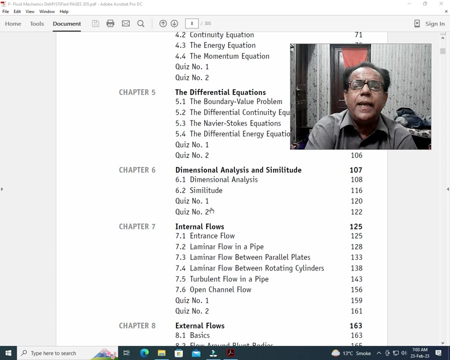 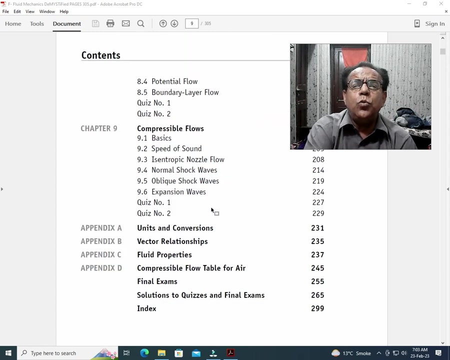 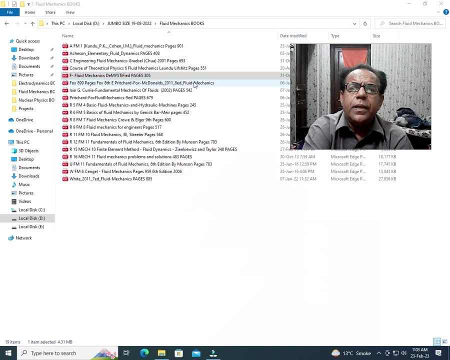 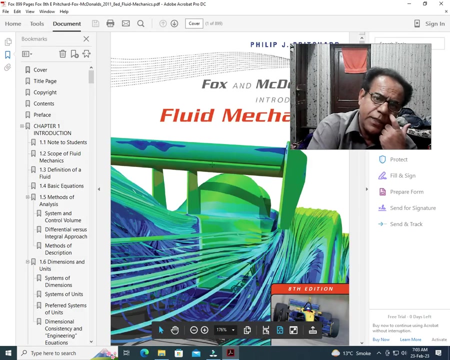 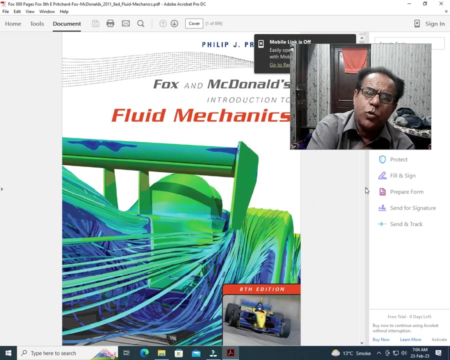 Okay, so we we confirm this. We confirm this thing. Okay. Yes, this is 10. Okay, the students say this is page number two and this is page number 14. Here 12 pages difference. Pages difference is coming. Anyhow, I had to emphasize that this numbering differs from numbering of a hard copy of this book. Okay. Fluid mechanics demystified. Okay, a self teaching guide. Fluid mechanics demystified. Fluid mechanics demystified. The author's name is Merle C. Porter, PhD. Okay, Macra Hill is its publisher. Okay. M-E-R-L-E Merle or Merle. Okay, M-E-R-L-E Merle C. Porter, PhD. Okay. Now we move to next. Okay, Macra Hill is its publisher and copyrights are of 2009. Okay. So this book was published in the year 2009. 2009. Okay. 2009. Now we come towards its contents. Okay. The essentials. Okay. The essentials. Fluid statics. Fluids in motion. Okay. The integral equations. The differential equations. Dimensional analysis and similitude. Okay. Internal flow. Internal flow. External flows. Compressible flows and indexes given at page number 299 of this book. Okay. Yeah. Take him on a metro. Next book consists of 899 pages, 899 pages as per soft arrangement. Okay. 899 pages in accordance with soft copy arrangement. Ok. Soft copy arrangement. 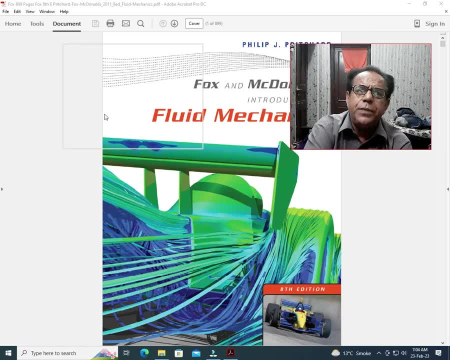 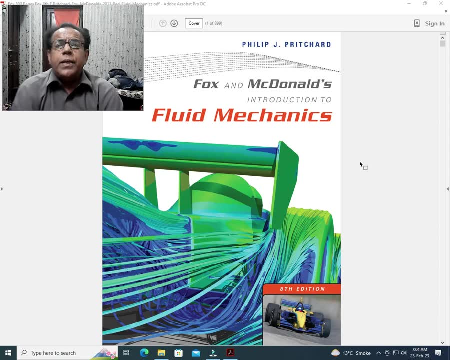 This is the picture. This is the situation. Philip J. Pritchard. Ok. 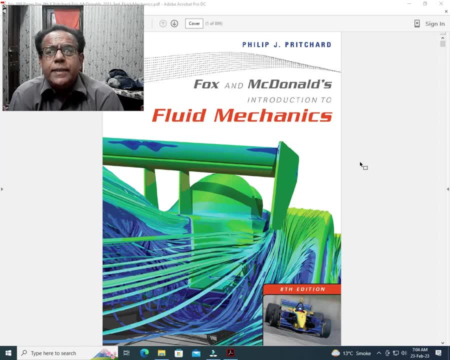 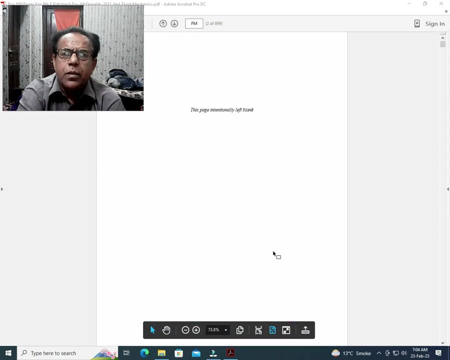 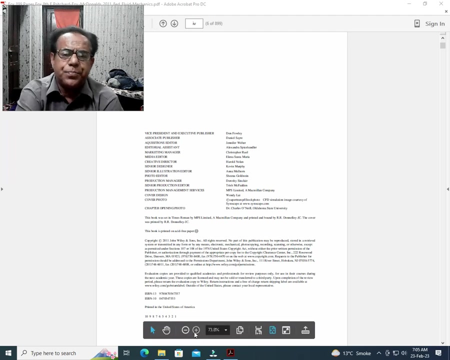 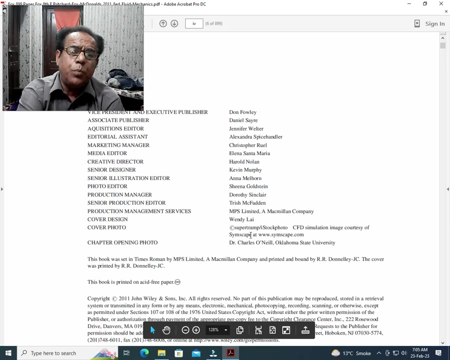 Philip J. Pritchard. I think Pritchard. Philip J. Pritchard. Philip J. Pritchard. Fox and McDonald's introduction to fluid mechanics. Okay. Fox and McDonald's introduction to fluid mechanics. Okay. Fox and McDonald's introduction to fluid mechanics. Eighth edition. Okay. Eighth edition. Philip J. Pritchard with special contribution from John. C. Lelygian. Lelygian. Lelygian. With special contribution from John C. Lelygian. Anyhow, John Wiley and Sons is its publisher. And now we see year of publication. Okay. Copyright 2011. 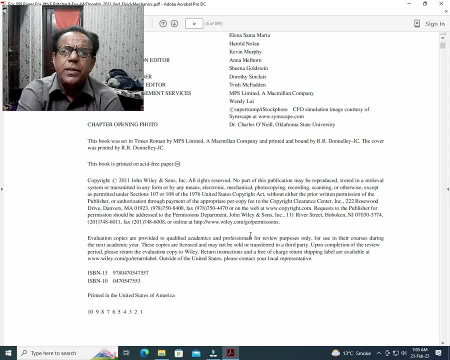 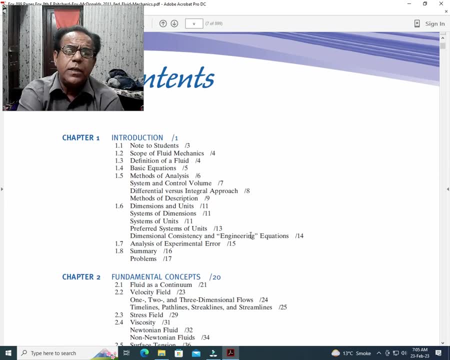 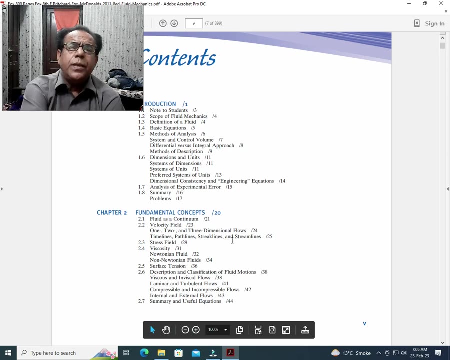 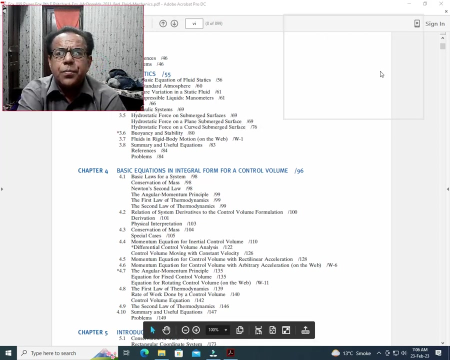 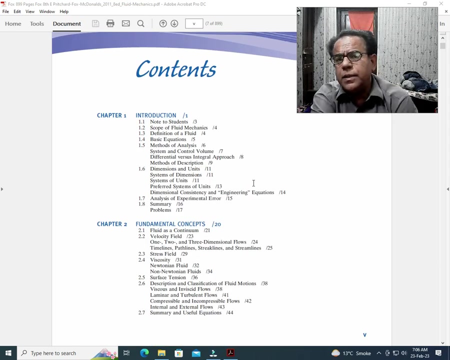 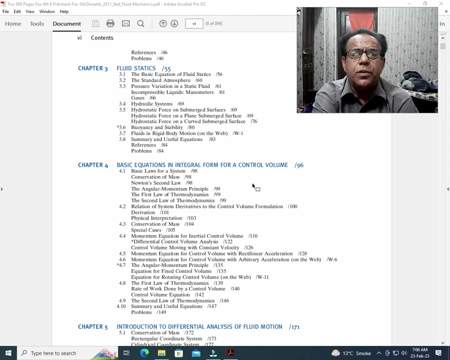 Years of previous editions will also be given at some place anyhow. We come towards contents. Okay. Introduction. Introduction. Introduction fundamental concepts. Introduction. Fundamental concepts. Fluid statics. Basic equations in integral form for a controllable volume. Okay. Introduction to differential analysis of fluid motion. 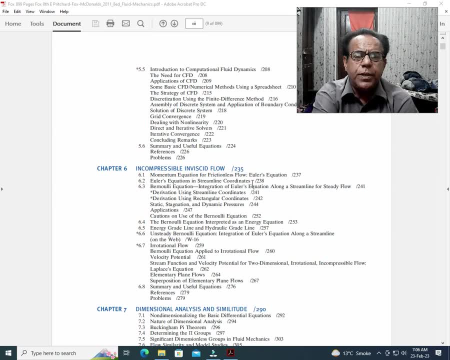 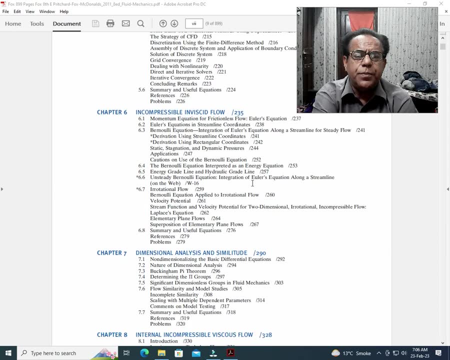 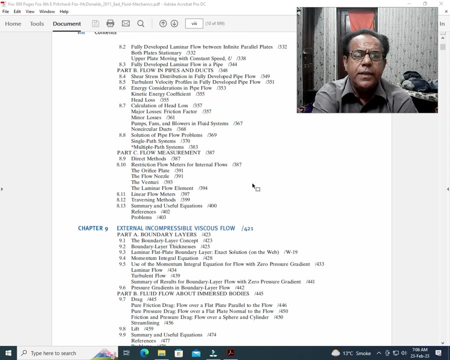 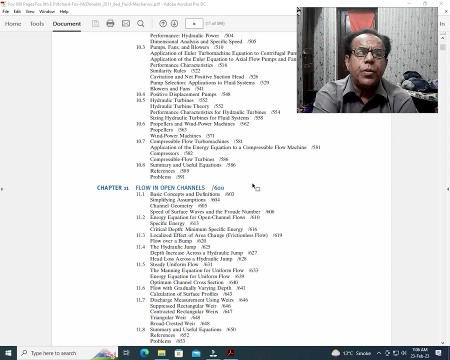 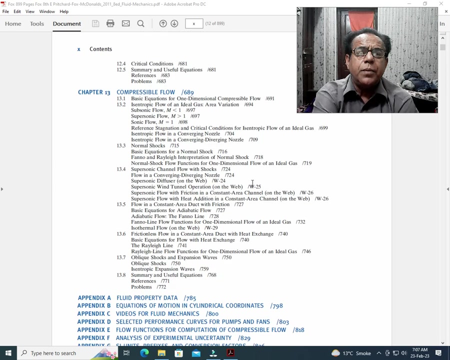 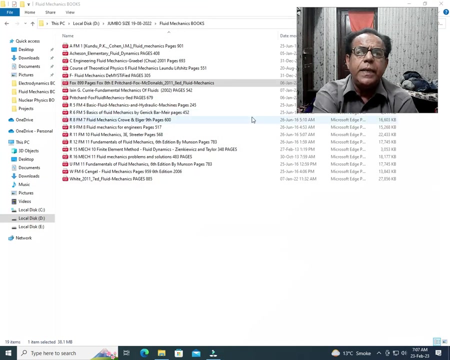 Incompressible in viscous flow. Dimensional analysis and similitude. Similitude. Internal incompressible viscous flow. External incompressible viscous flow. Fluid machinery. Flow in open channels. Introduction to compressible flow. Compressible flow. Okay. Then index is given at page number 867. Okay. 867. And next book. 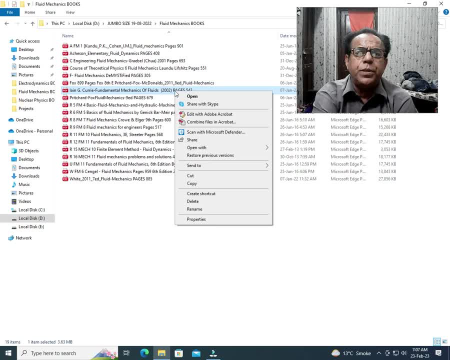 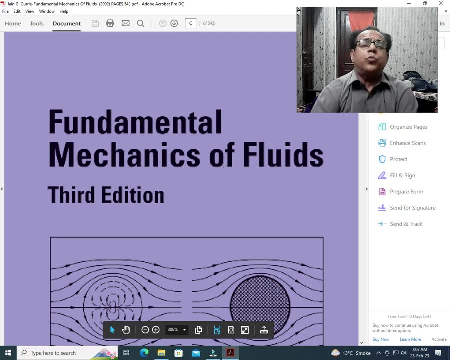 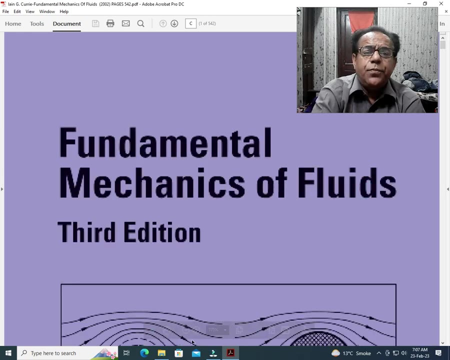 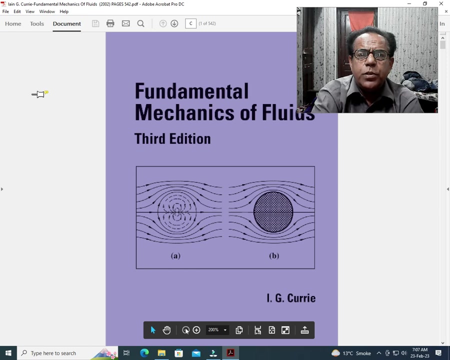 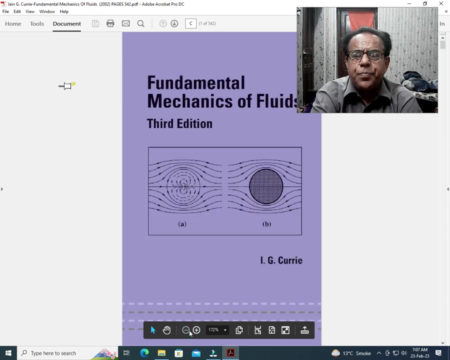 consists of 542 pages ok 542 pages this book consists of 562 pages as per soft format okay fundamental fundamental mechanics of third edition I G Q E I G U D fundamental mechanics of third edition I G Q E I G Q E fundamental mechanics of third edition I G Q E 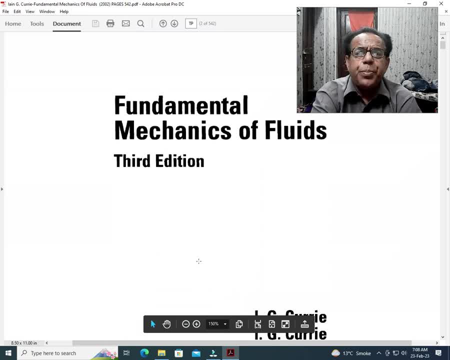 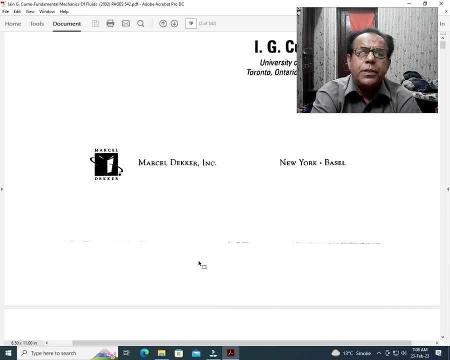 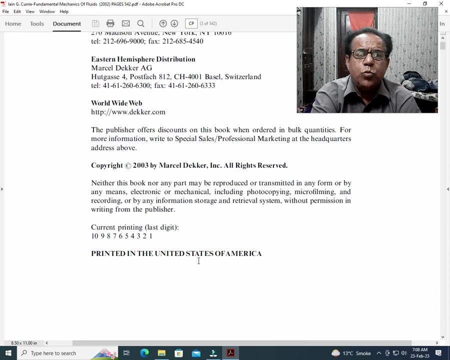 fundamental mechanics of rules the third edition I G Q E its publisher is Marcel Decker Marcel Marcel Decker this publisher has appeared first time in our collection of books of a copyright 2003 okay so this book was published in the year 2003 you 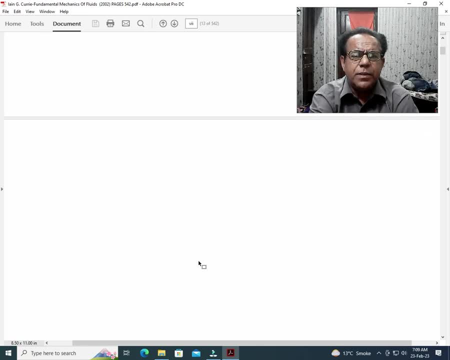 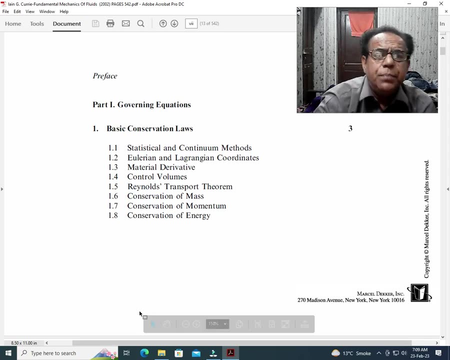 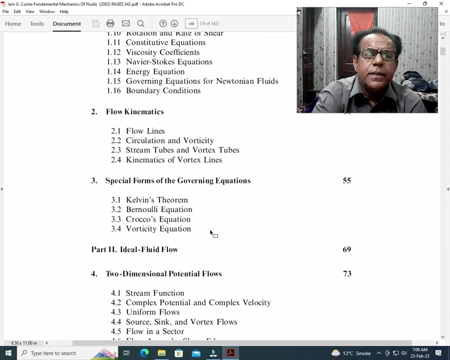 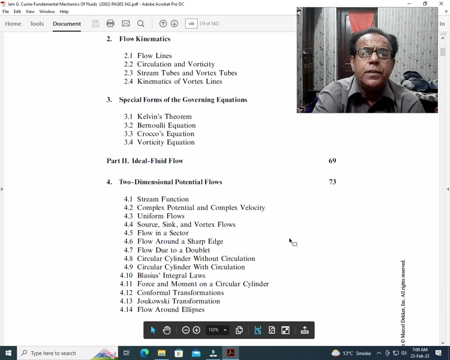 , preface not here mentioned okay now contents okay governing equations basic conservation laws flow kinematics special forms of governing equations special forms of governing equations ideal fluid flow this is part second okay from here second part begins 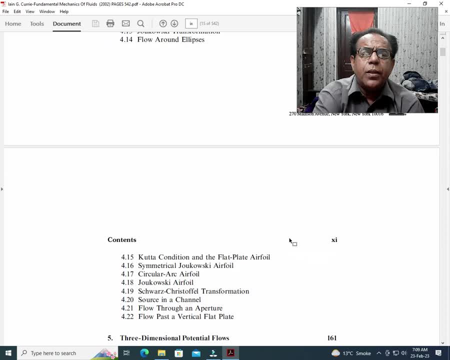 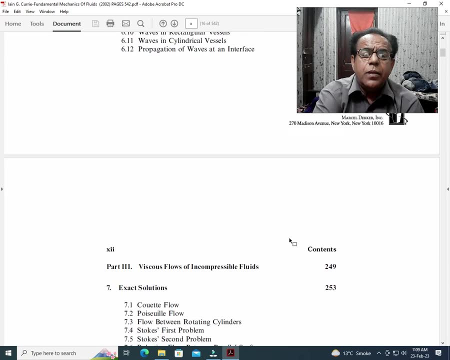 this reading I did dimensional potential flows three dimensional potential flows surface waves exact solutions the low Reynolds and 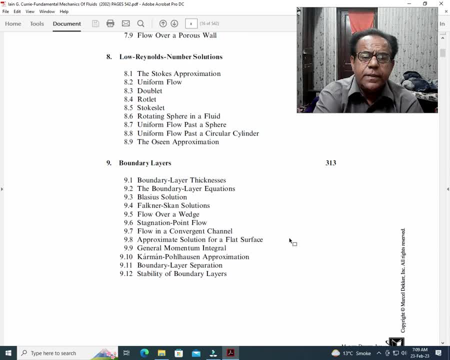 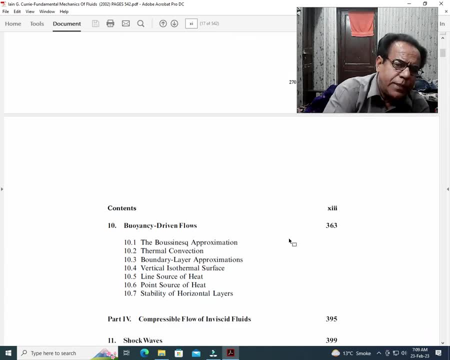 number solutions boundary layers buoyancy-driven flows compressible flow off in Inviscid fluids 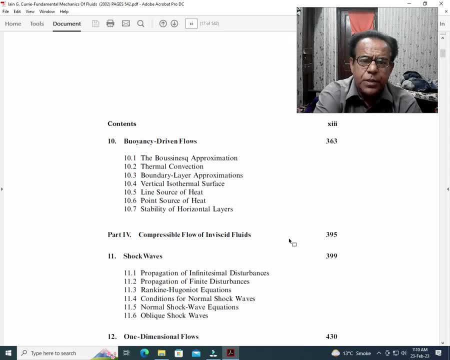 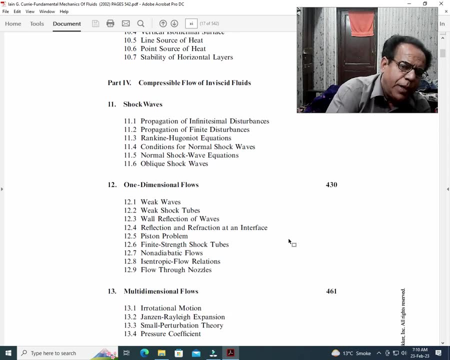 This is from here. Fourth part of this book begins. Shock waves, 11th chapter, one-dimensional flows, multi-dimensional flows and then index is given at page number 521. 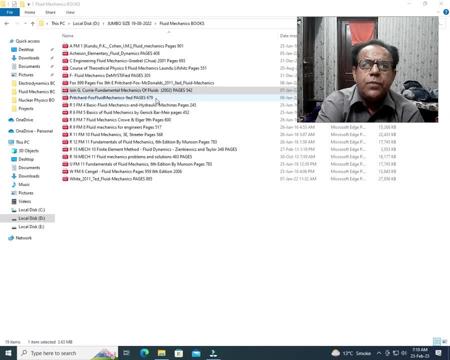 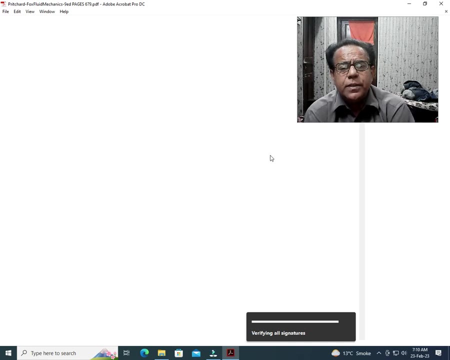 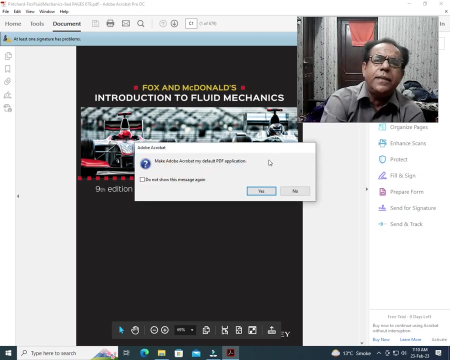 Okay, 521. Next book consists of 679 pages. Okay, 679 pages. Yes, this is the book consisting of 679 pages. This is again almost previous. 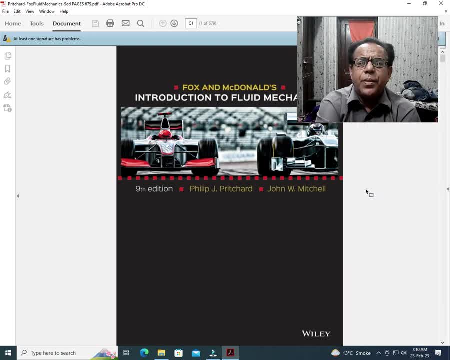 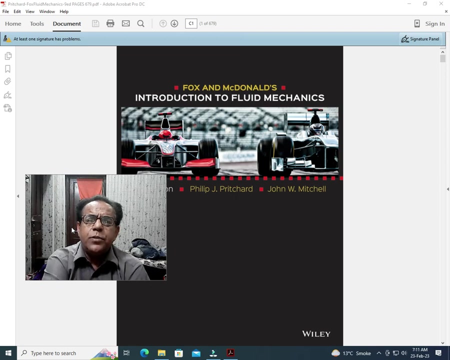 I don't know, perhaps it's different. Yeah, edition may be different. Otherwise, similar situation has already been gone through by us. Okay, Fox and McDonald's introduction to fluid mechanics. Okay, Fox and McDonald's introduction to fluid mechanics. Ninth edition. 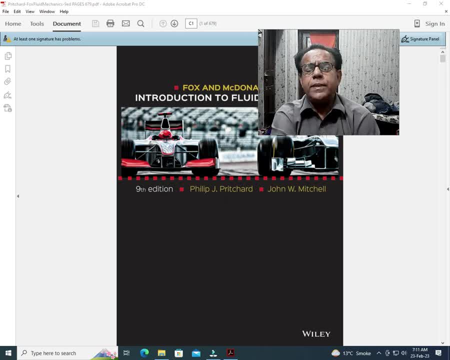 Philip J. Pritchard. Okay, this author has been previously used, but this is new author. Okay, because this edition is next ninth edition. 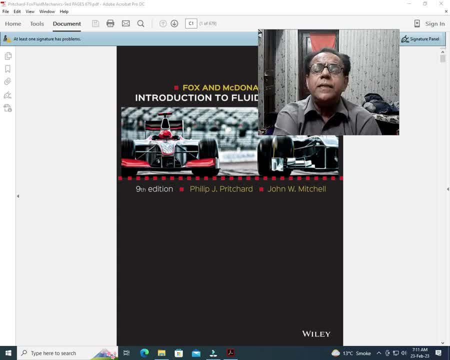 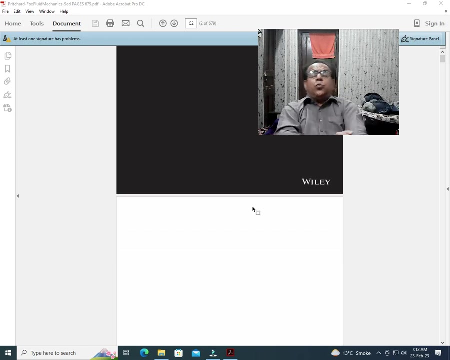 So definitely this may be the original author and in subsequent editions, sometimes in case of death of original author. And some co-author appears from some corner to run that business smoothly. Okay, so publishing books definitely is a business. Okay, so Baile is the publisher of this book. 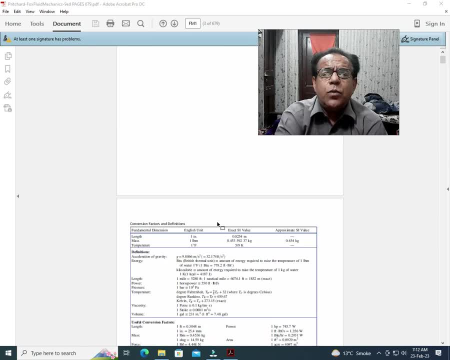 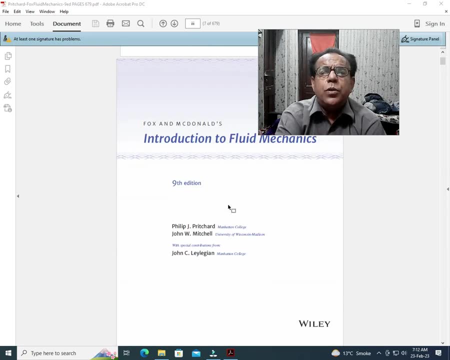 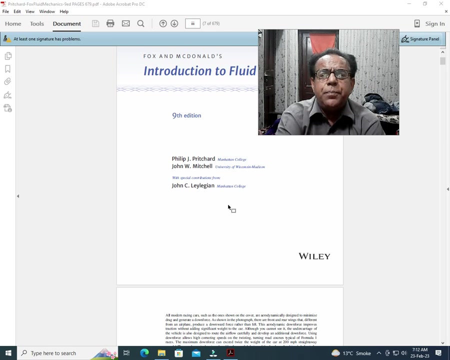 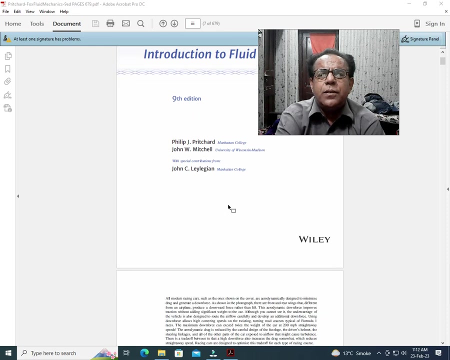 And now we come towards its contents. Okay. Contents Fox and McDonald's introduction to fluid mechanics. Ninth edition. Philip Pritchard and John W. Mitchell. Another name is given special contribution from John C. Lilligian. Okay, this was also available in previous edition, but this name is new. Okay. Here are some last fertilizers. John W. Mitchell. 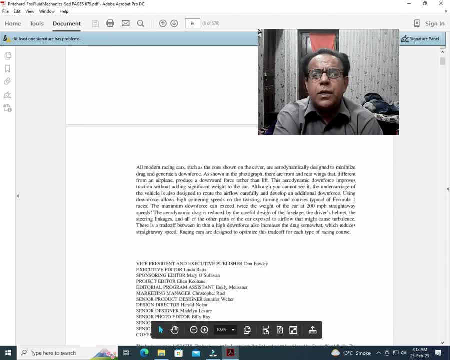 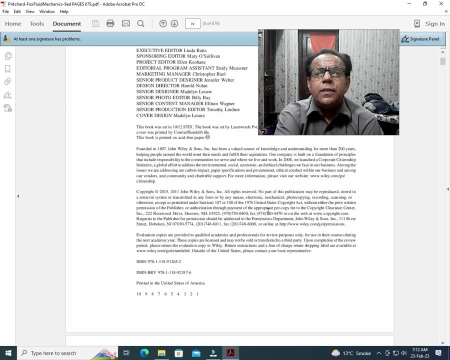 Now, we come towards its years of publication, okay. Now, we come towards its years of publication. Okay. The years of publication, yes. The years of publication... 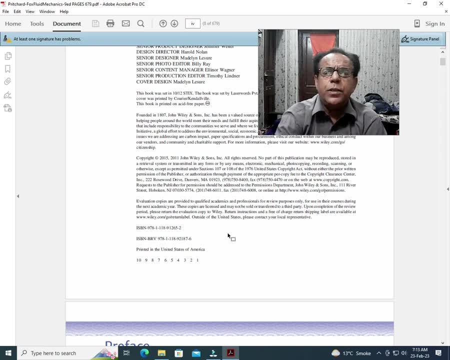 Yes, the copy right was 2015 and the previous edition was in 2011. Okay. Presently only two years are given, 2011 and 2015. Okay. Presently only two years are given, 2011 and 2015. Okay. 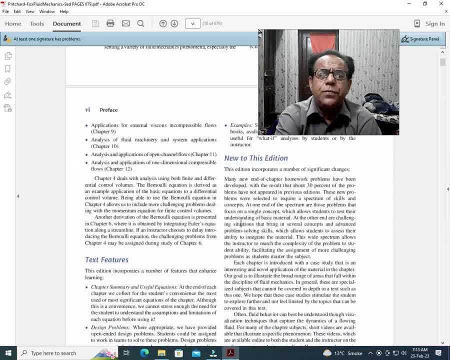 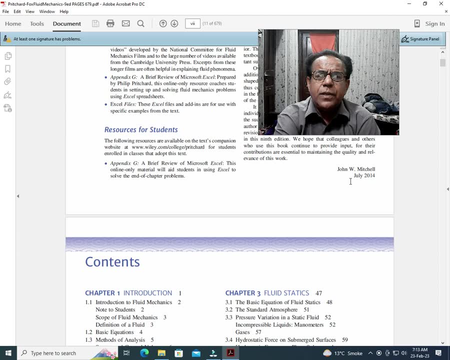 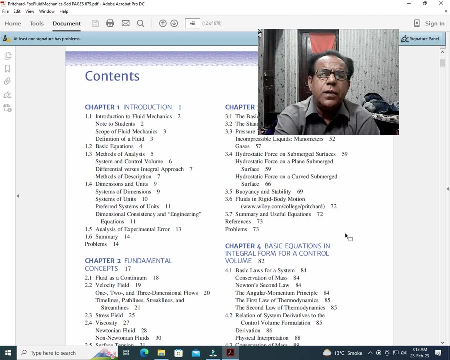 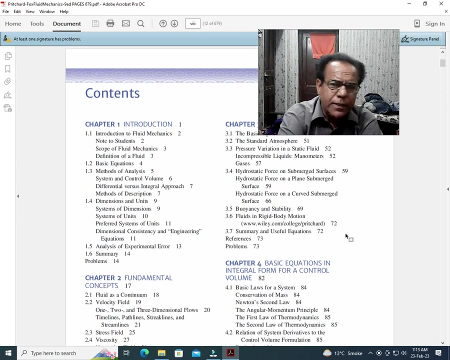 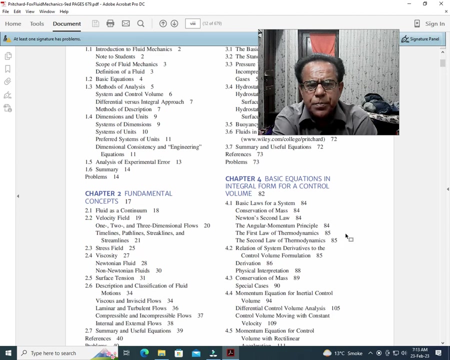 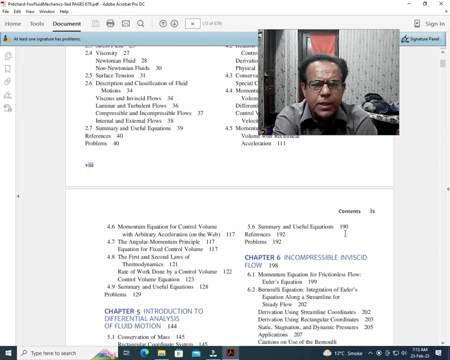 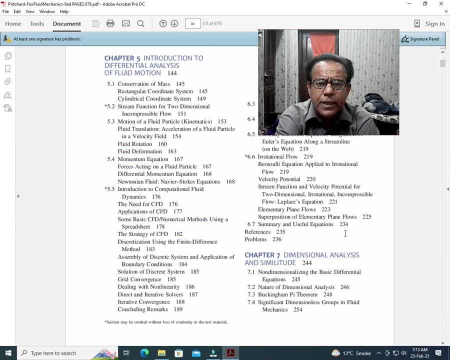 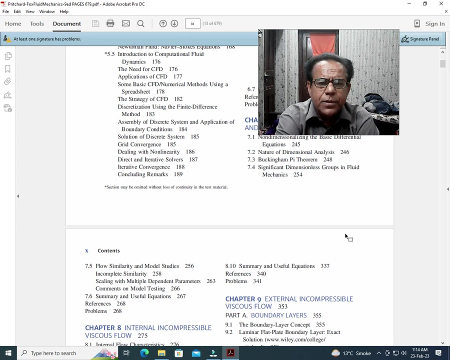 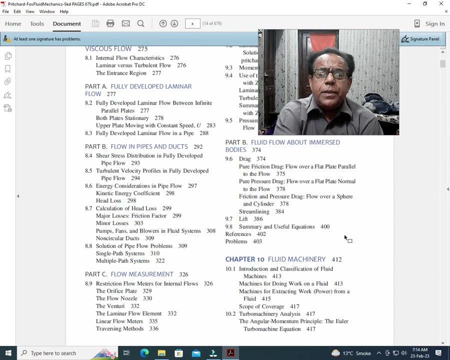 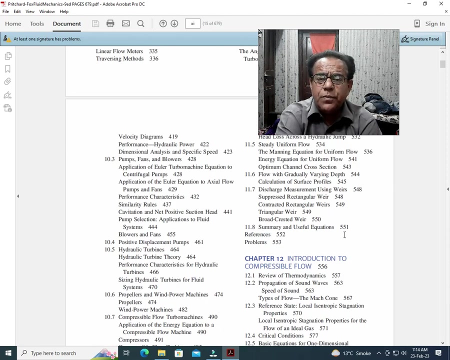 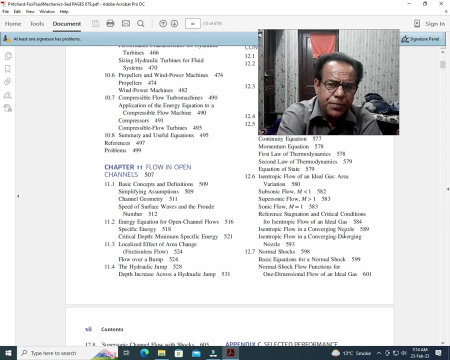 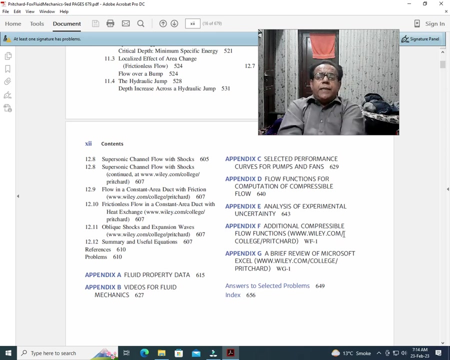 means this edition was published in 2015 and now we come towards contents okay its preface was written in the in july 2014 contents okay introduction chapter number one introduction while chapter number three fluid statics chapter number two fundamental concepts chapter number four basic equations in integral form for a control volume okay chapter number six incompressible in biscuit flow chapter number five introduction to differential analysis of fluid motion chapter number seven dimensional analysis and similitude chapter number eight internal incompressible viscous flow chapter number nine external incompressible viscous flow chapter number ten fluid machinery of chapter number twelve introduction to compressible flow chapter number eleven flow in open channels and then appendix index is given at page number 656 okay index of this book is given at a page number 656 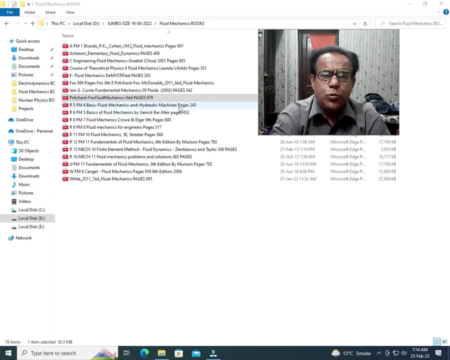 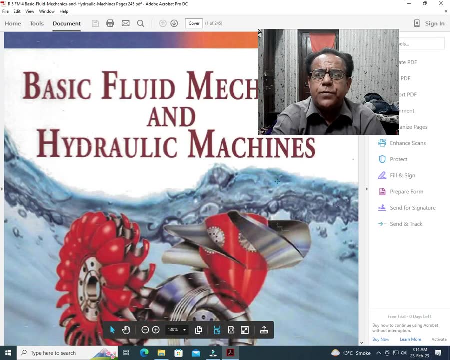 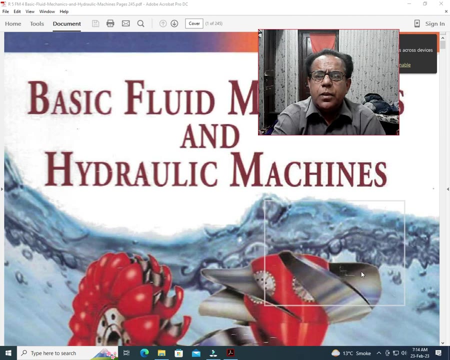 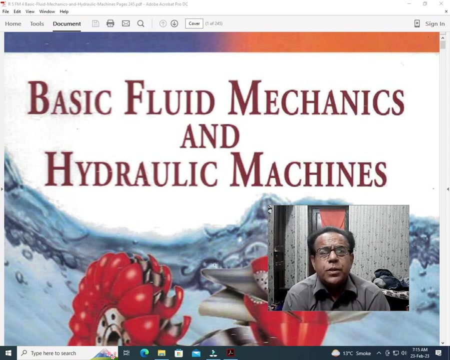 So, next book consists of 245 pages, next book consists of 245 pages, okay, 245 pages, relatively small size book, okay, we should emphasize on quality rather than quantity, okay, basic fluid mechanics and hydraulic machines, okay, 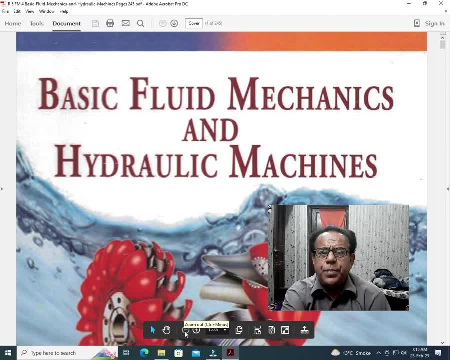 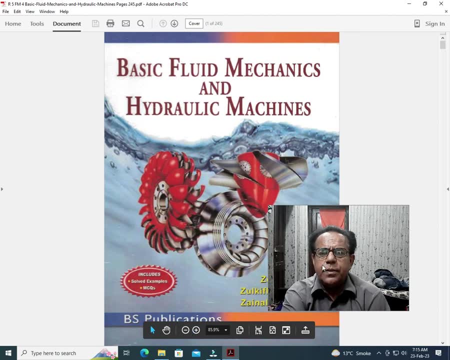 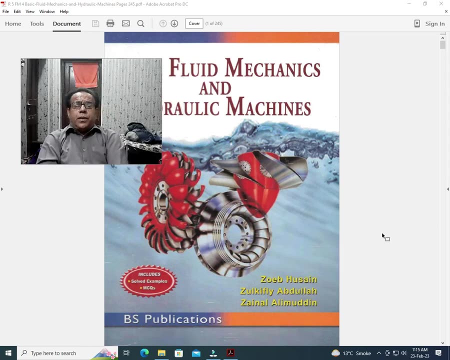 okay, basic fluid mechanics and hydraulic machines, yes, when we reduce its size, then other things become visible, its authors are Zoyaib Hussain, okay, definitely this is a Muslim author, but it may belong to some other country, here in Pakistan, 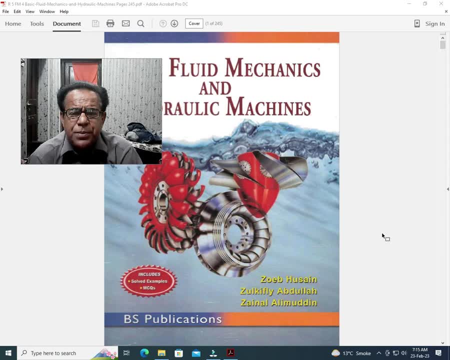 Zoyaib does not appear in such, with such spelling, okay, anyhow, Zoyaib Hussain, Zulkiflai Abdullah, this is again Muslim, but Zulkiflai is a very unusual name, then Zainal Alimuddin, this is slightly similar to Pakistan, Pakistani Muslim names, okay, Zainal Alimuddin, Zainal Alimuddin, okay, all the three writers are Muslim authors, but despite this, their names are very different from Pakistani Muslim names, okay, anyhow, we have nothing to do from, we have nothing to take from names, 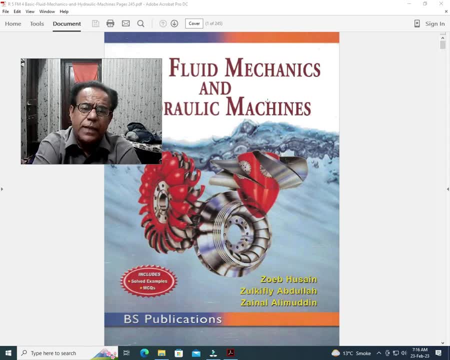 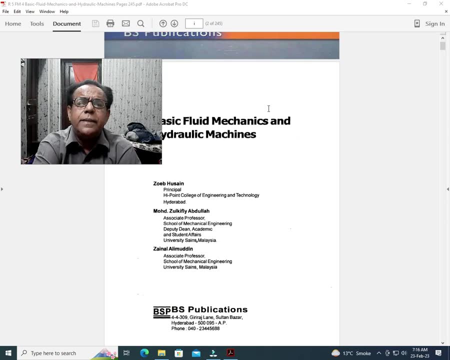 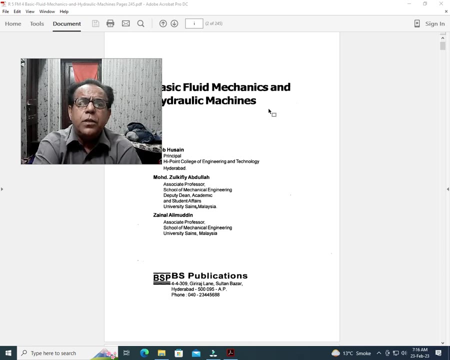 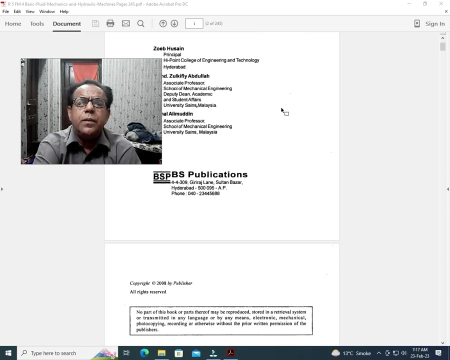 okay, we have to take only from contents, BS Publications is the publisher, okay, basic fluid mechanics and hydraulic machines, Zyaib Hussain, Mohd, Mohamad, Zulkiflai Abdullah, Zainal Alimuddin, this is the publisher, copywriter 2008, 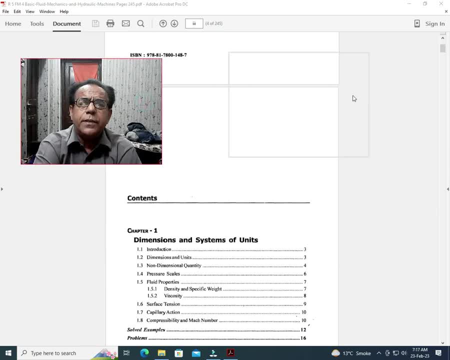 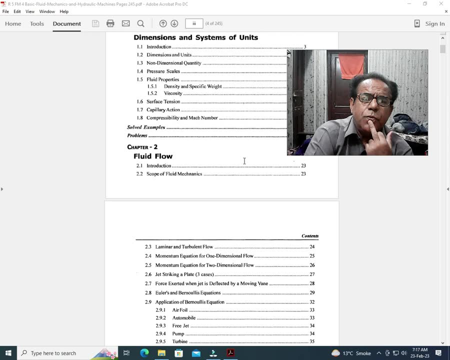 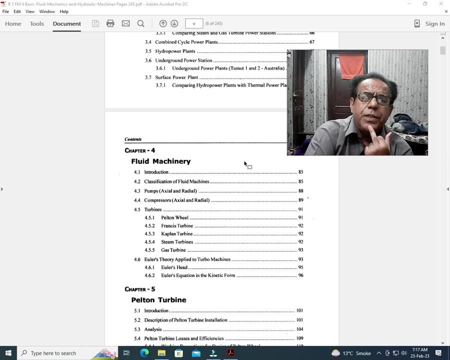 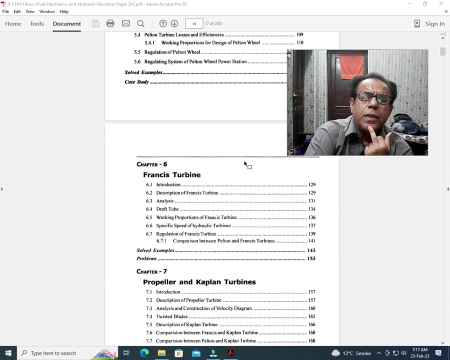 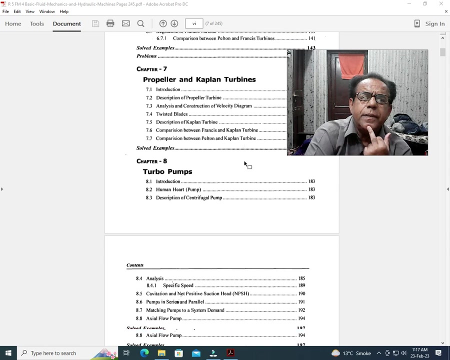 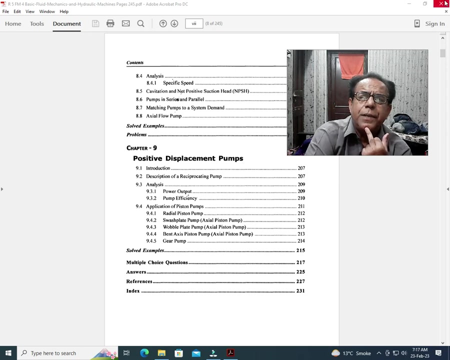 2008 copyright, now we come towards its contents, okay, yes, contents are important, dimensions and systems of units, fluid flow, thermal and hydropower stations, machinery, fluid machinery, turbine, Pelton turbine, okay, Frankish turbine, propeller and Kaplan turbines, turbo pumps, positive displacement pumps, index is given at page number 231, next book consists of 452 pages, 452 pages, 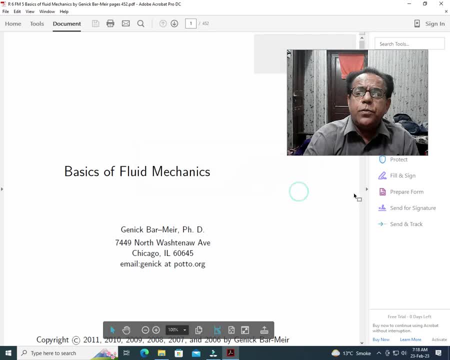 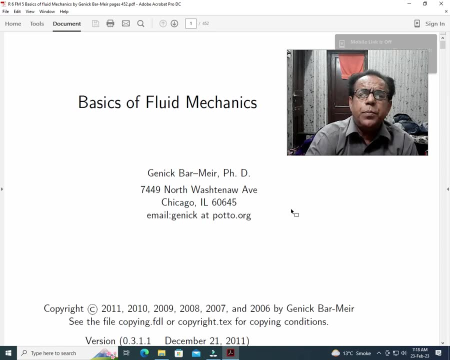 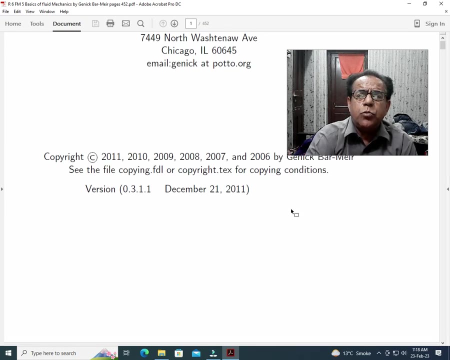 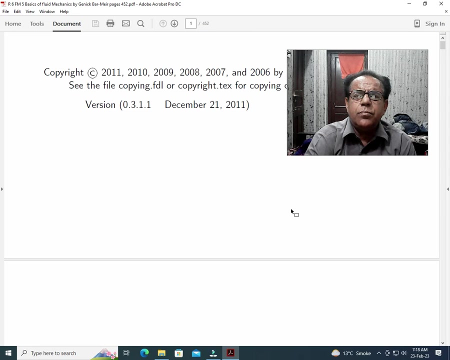 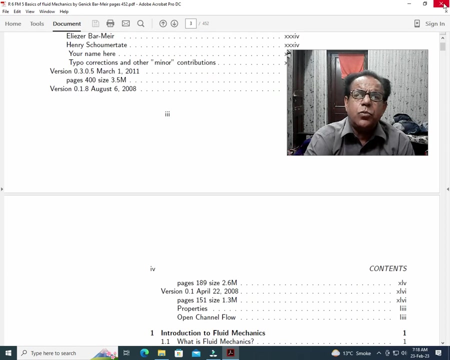 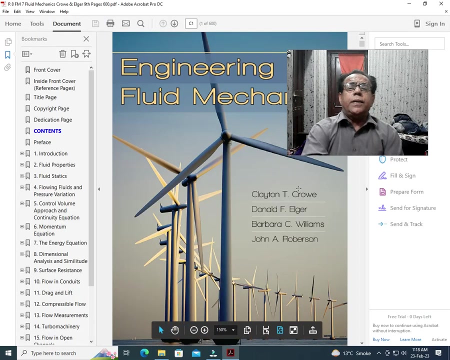 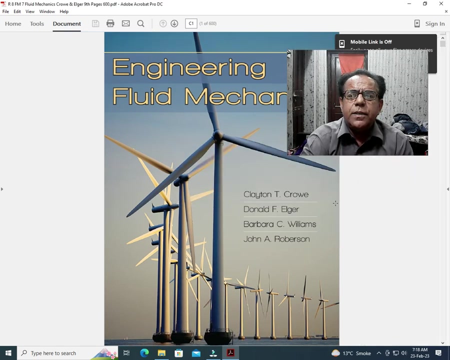 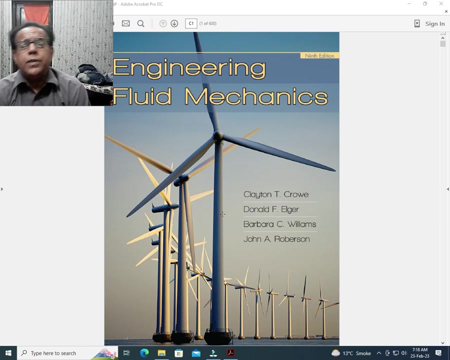 okay, next book consists of 452 pages, okay, basics of fluid mechanics, Chicago, copyright 2011, previous editions, 2006, 7, 8, 9, 10, 11, version December 21, 2011, subdivision담 3, I believe this book, okay, next book consists of 600 pages, next book consists of 600 pages, and very dashing appearance, definitely, it may be assumed very important book, okay, 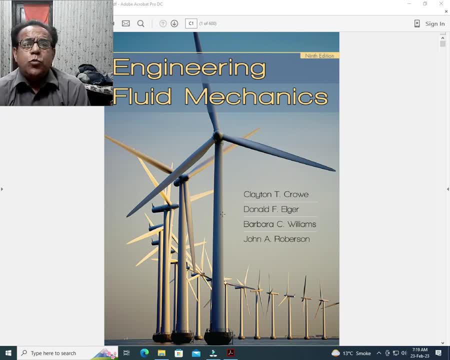 Ninth edition, Engineering Fluid Mechanics, it has four authors, okay, C-L-A-Y-T-U-N, Clayton T. Crowe, C-R-O-W-E, okay, Donald F. Elgar, Barbara C. Williams, John A. Roberson, Roberson, Roberson, Roberson, Roberson, John A. Roberson, okay. 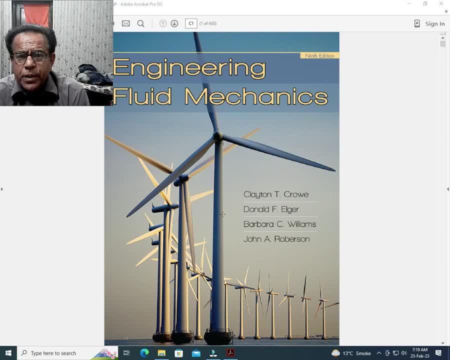 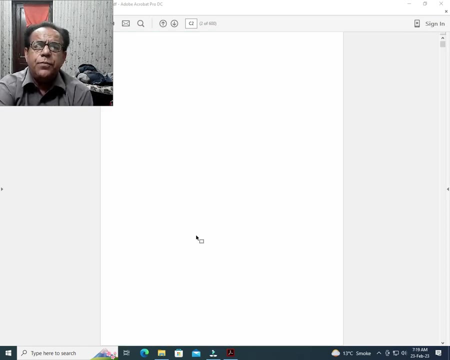 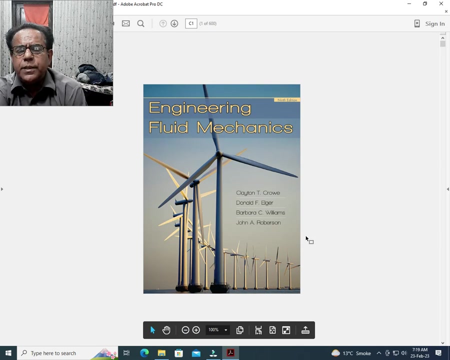 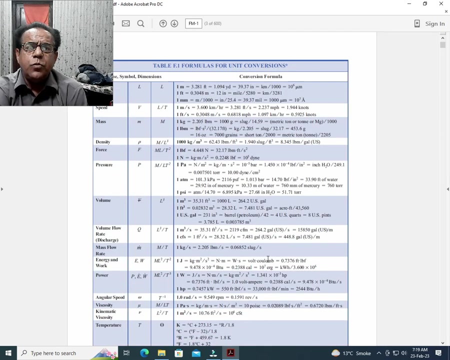 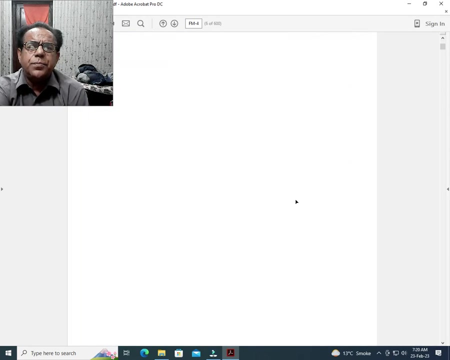 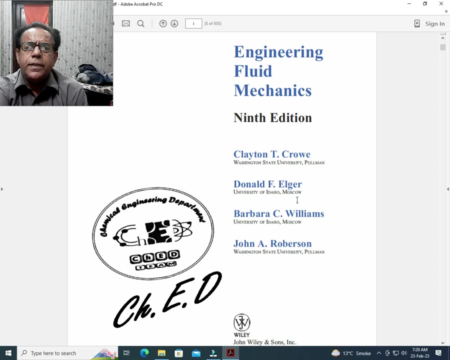 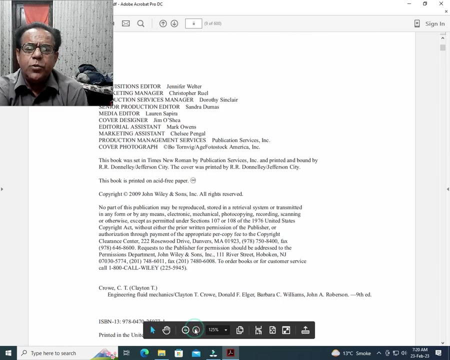 And once again, I try to pronounce this, Clayton T. Crowe, Donald F. Elgar, Barbara C. Williams, John A. Roberson, okay. We move forward, but before moving forward, we, okay, yes, now complete page is shown. Okay. We are going to its contents. Engineering Fluid Mechanics, ninth edition, okay, Clayton T. Crowe, Donald F. Elgar, Barbara C. Williams, John A. Roberson, Wiley, John, John Wiley Edsons is the publisher of this book, and now we see here's the publisher. 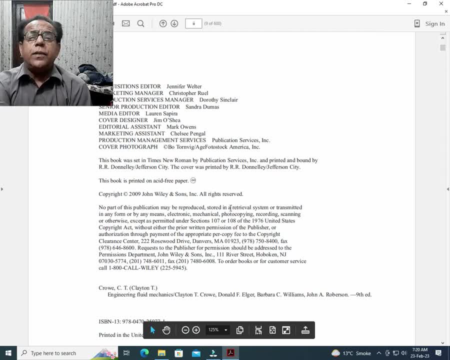 okay 2009 okay this book was published in the year 2009 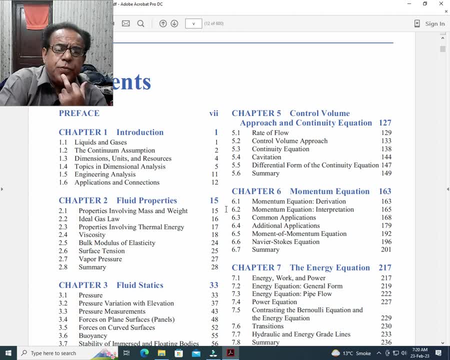 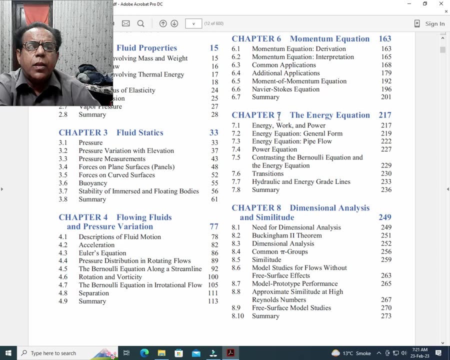 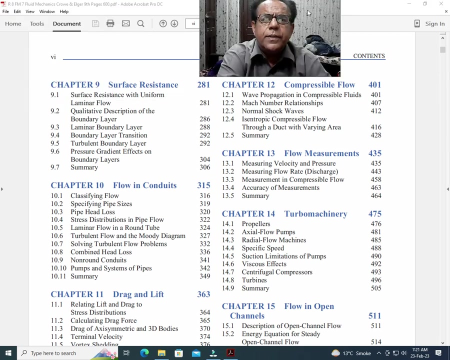 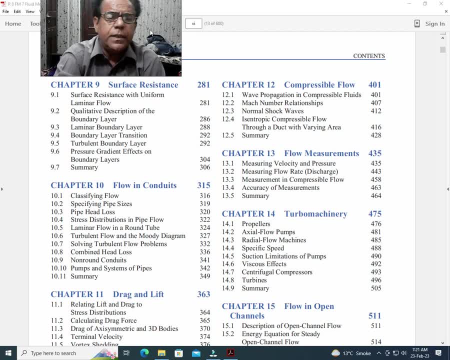 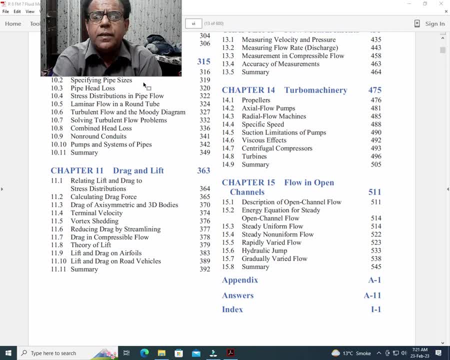 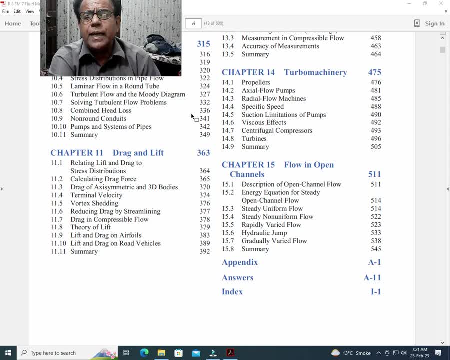 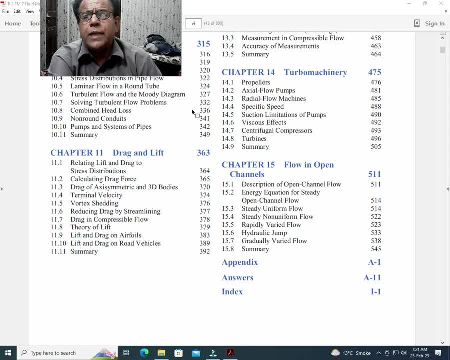 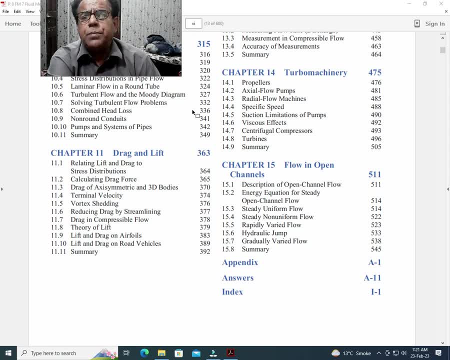 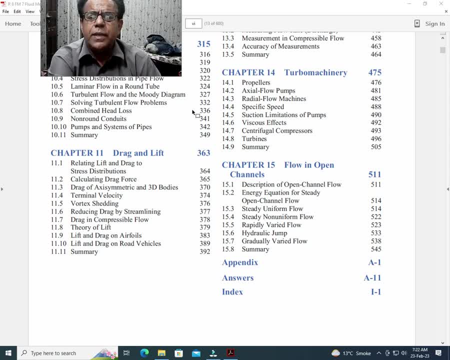 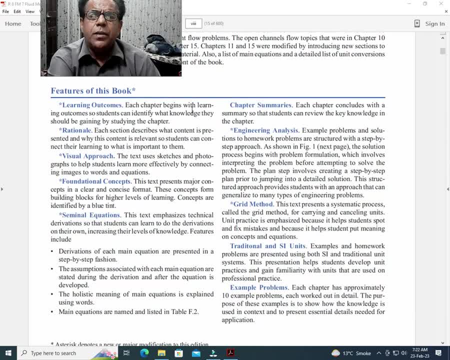 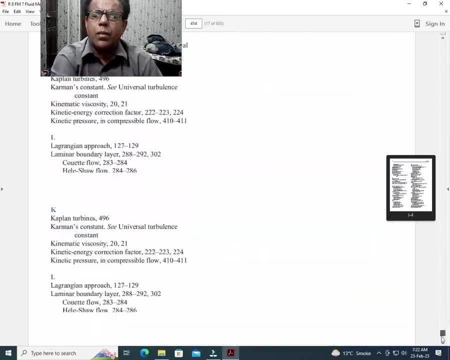 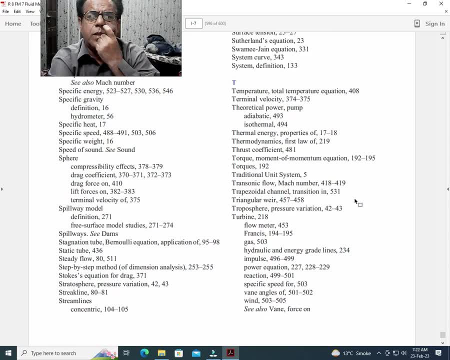 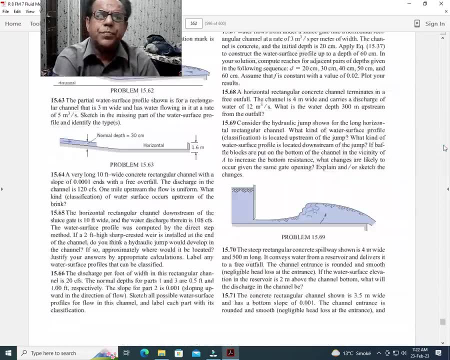 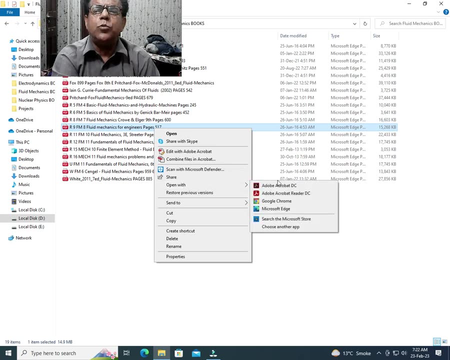 next book consists of 5 517 pages okay 517 pages 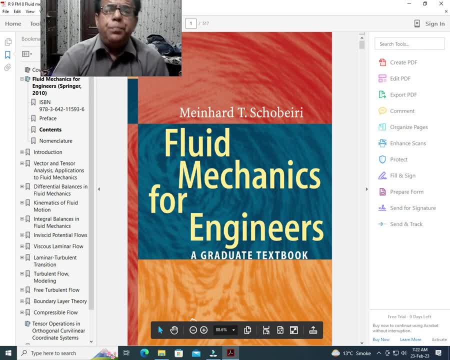 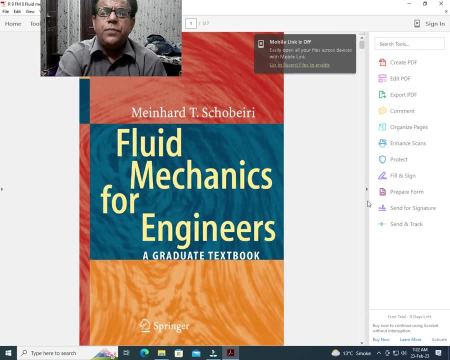 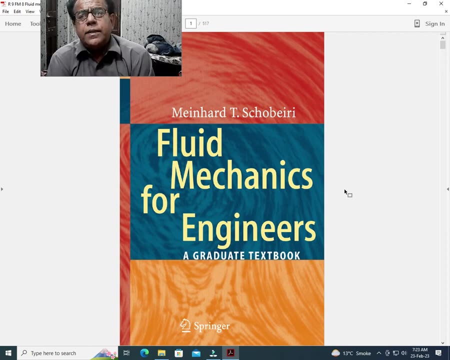 mean hard to show very okay if his a show very then what I can do mean hard to show Brie okay and me and me me and me and me and me in herd he is 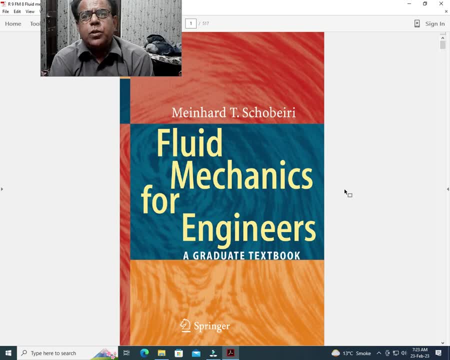 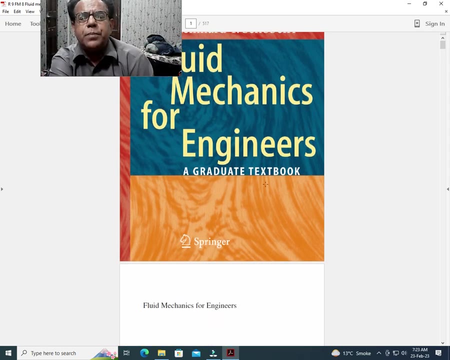 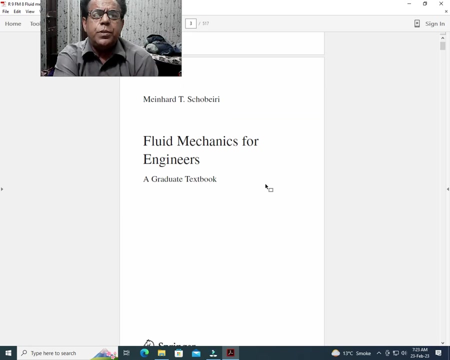 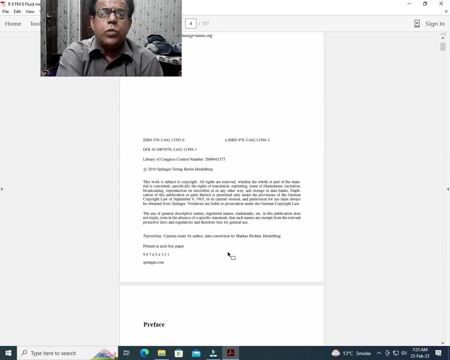 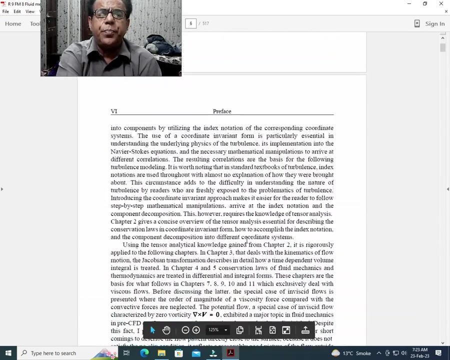 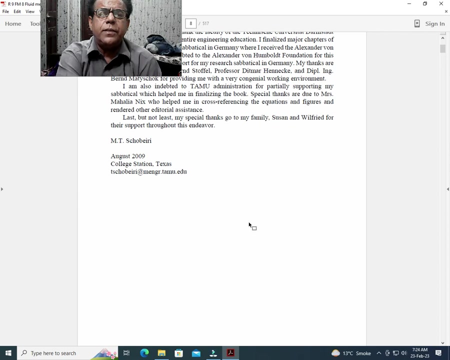 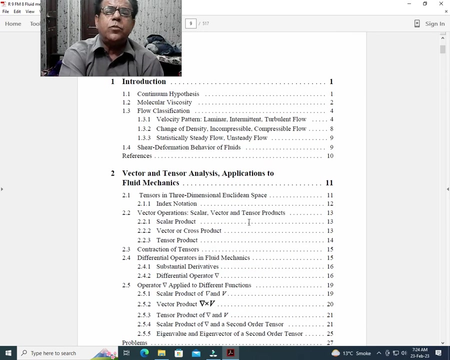 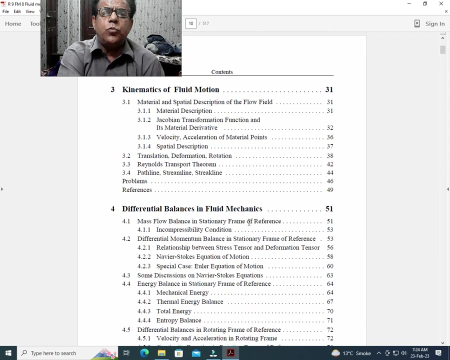 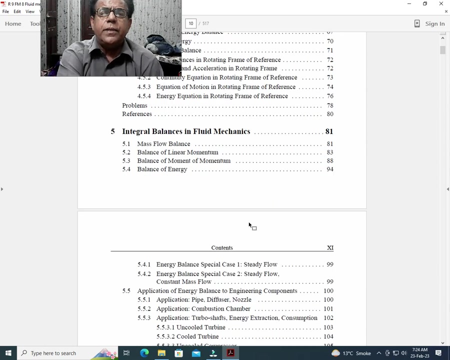 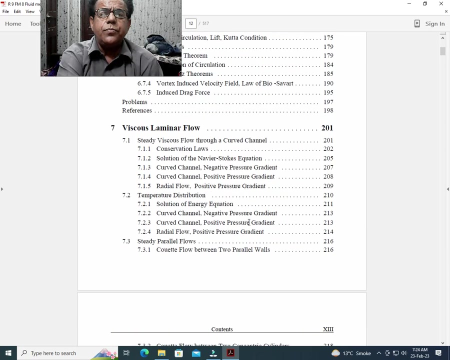 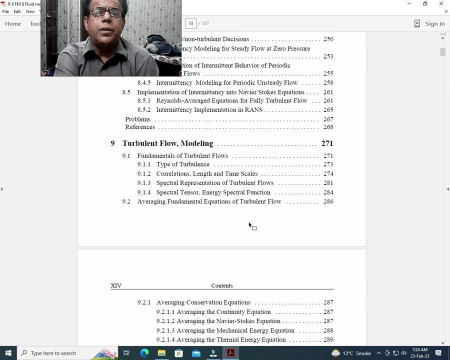 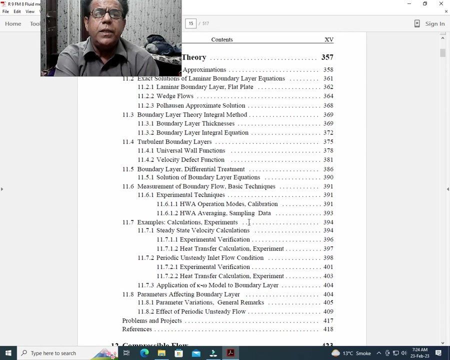 S-C-H-O-B-E-I-R-I, Shobri, okay, Meinhard T. Shobri, Meinhard T. Shobri, Meinhard T. Shobri, Fluid Mechanics for Engineers, a graduate text, Springer is its publisher, okay, Meinhard T. Shobri, Fluid Mechanics for Engineers, a graduate text, Springer is its publisher, Shobri, 2010, this book was published in the year 2010, okay, 2010, accordingly, preface was written in August 2009 by N.T. Shobri, okay, contents, introduction, vector and tensor analysis, applications to fluid mechanics, kinematics of fluid motion, differential balances in fluid mechanics, integral balances in fluid mechanics, in whisked flows, viscous laminar flow, laminar turbulent transition, turbulent flow modeling, free turbulent flow, boundary layer theory, compressibility, 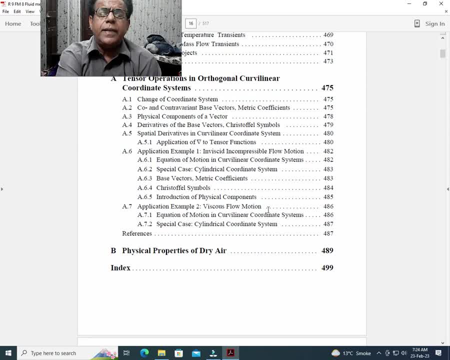 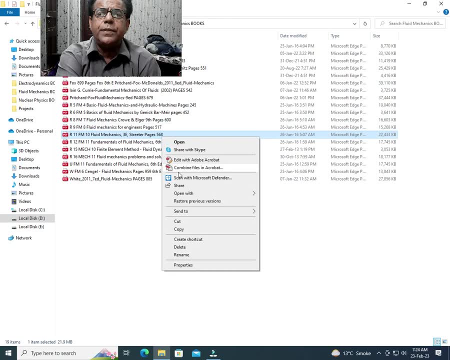 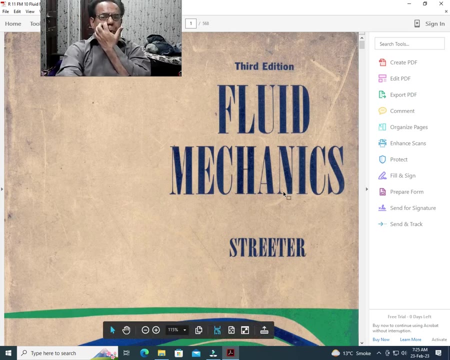 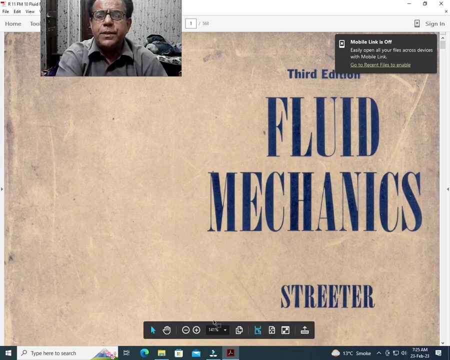 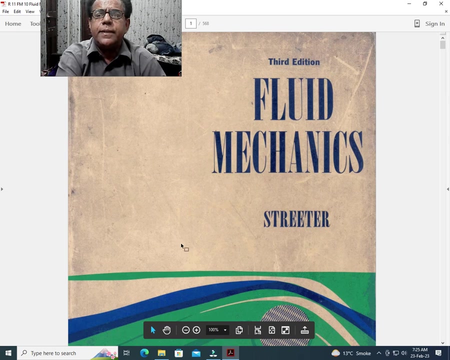 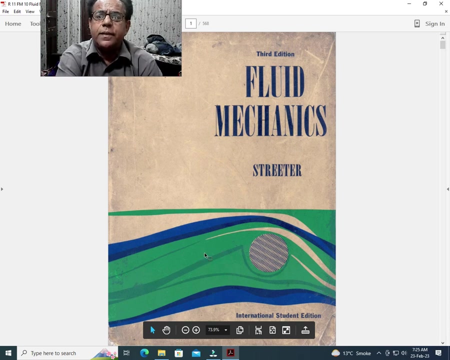 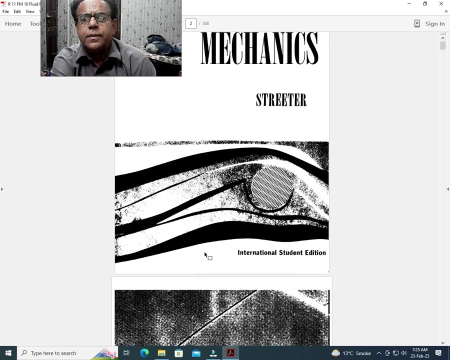 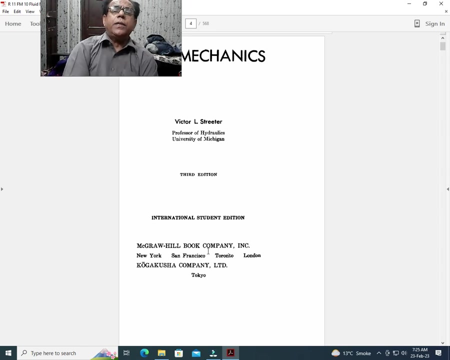 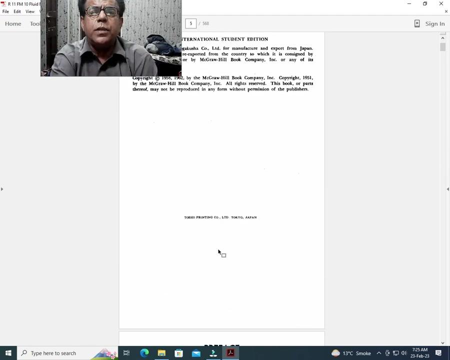 flexible flow, and index is given at page number 499, 499, next book consists of 568 pages, okay, next book consists of 568 pages, this is, okay, 568 pages, 568 pages, third edition, fluid mechanics, setreeter, S. E. Tr., this is easier name, okay, third edition, fluid mechanics, setreeter, S. Tr., third edition, fluid mechanics, 음악, Hampus Kalak, Vermilion Crosswind, życie, British타 mingue, et lancome keiderman, aus dialectis, ediketalit, et lancome, et lage für die, Macra Hill is its publisher. Copyrights 1958 and 1962. 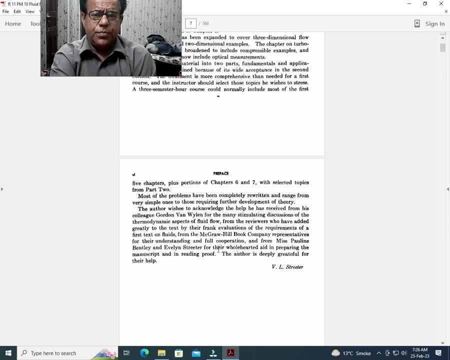 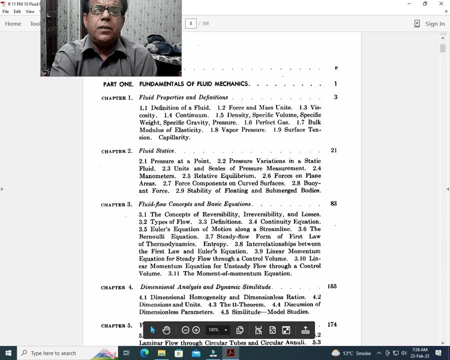 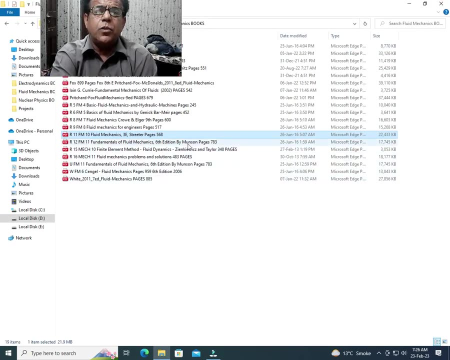 Contents. Dear students, I am leaving contents. Contents will be similar to previous contents. 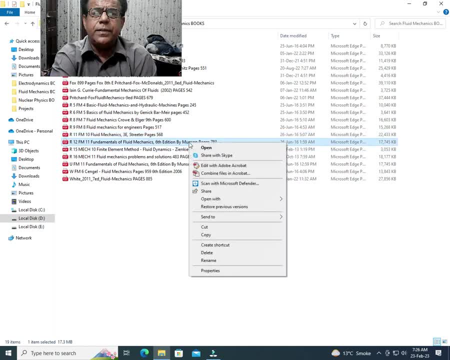 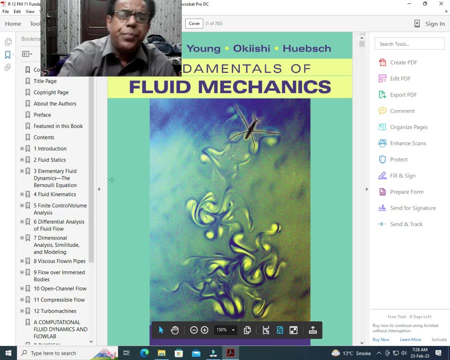 Next book consists of 783 pages as per soft format. 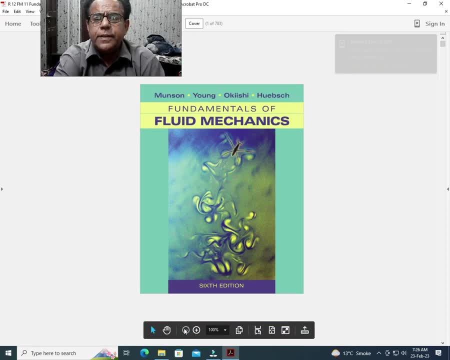 This is 6th edition. 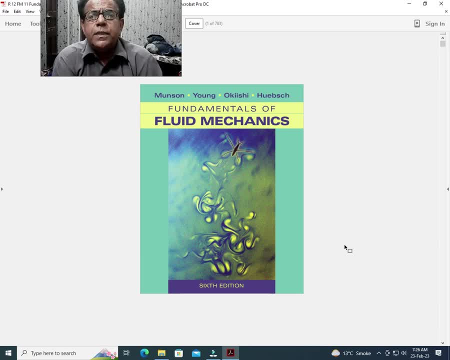 Mansand, Young, Okilishi, Hubesh. So dear students, if he is Hubesh then what I can do? I can do nothing. 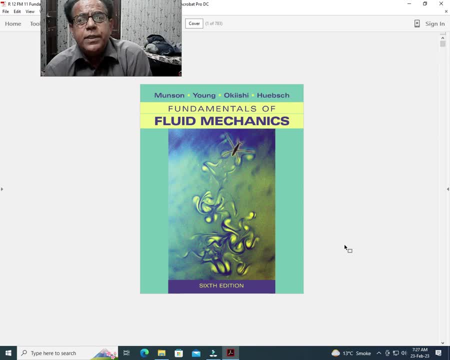 Mansand, Young, Okilishi, Hubesh. Fundamentals of Flow Mechanics, 6th edition. 6th edition. 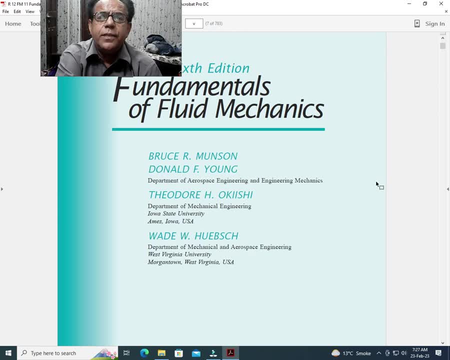 6th edition. Fundamentals of Flow Mechanics. Bruce R. Manson. 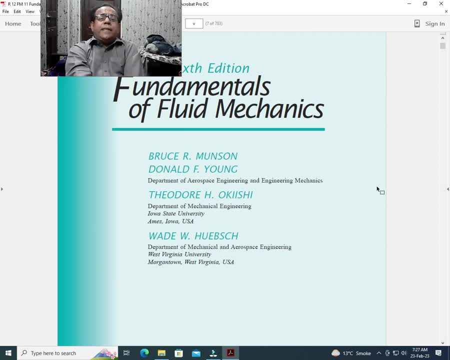 The only difference is that here full names are given. In first page, names in relatively short manner were given. In first page, names in relatively short manner were given. But here full names are given. 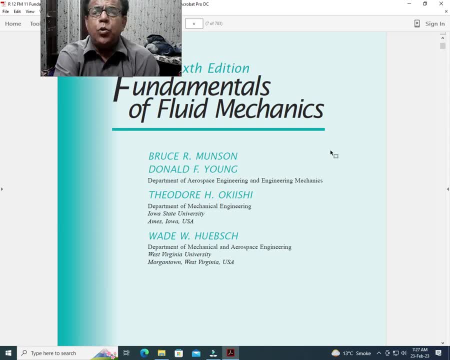 Bruce R. Manson. Donald F. Young. 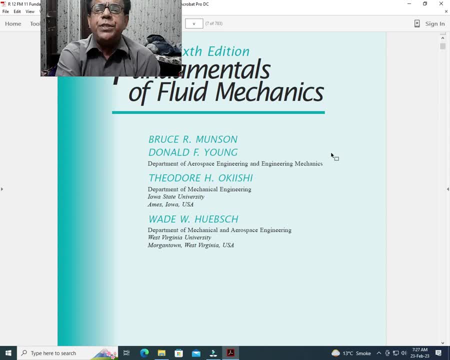 Theodore H. Okilishi. Wade W. Hubesh. 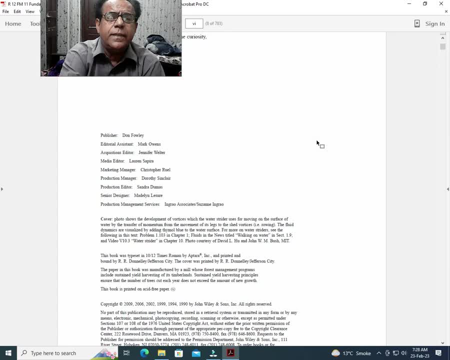 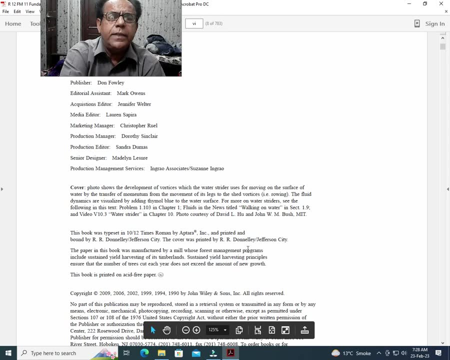 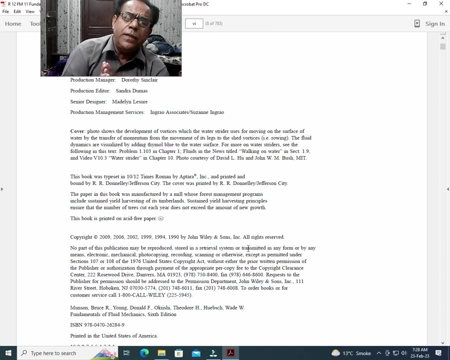 John Wiley & Sons is its publisher. And now we see year of publication. 2019. Its years of publication are given in descending order. But we will read in ascending order. 1990. 1994. 1999. 2002. 2006. 2009. 2006. 2005. 2013. 2004. 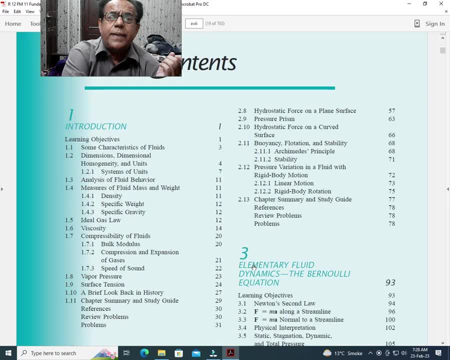 2005. 2003. 2005. 2006. 1994. 2000. 2003. 2009. 2005. tercer. 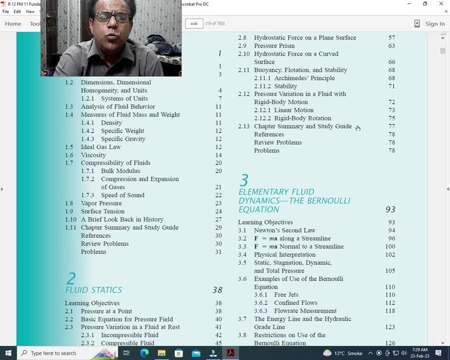 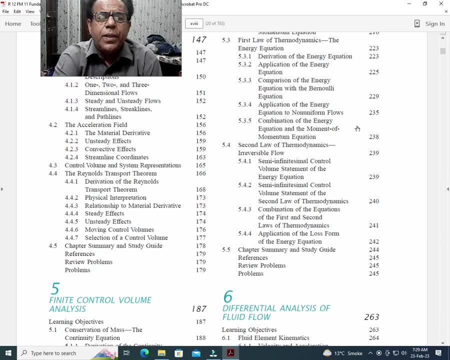 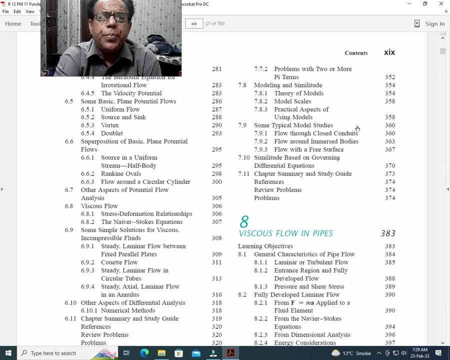 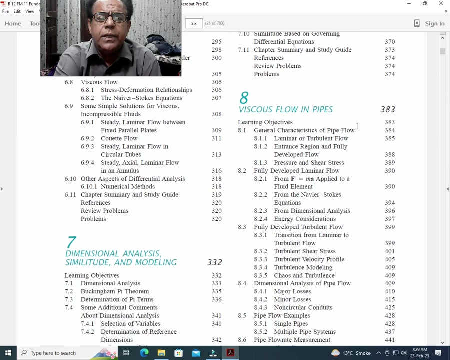 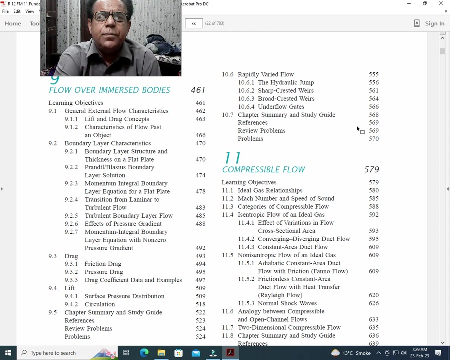 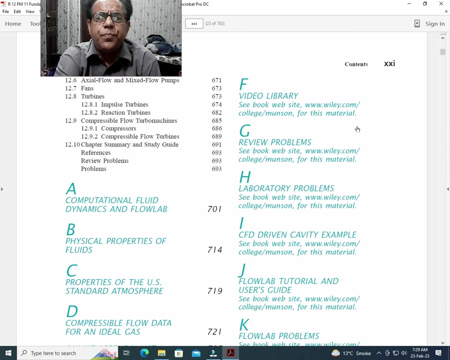 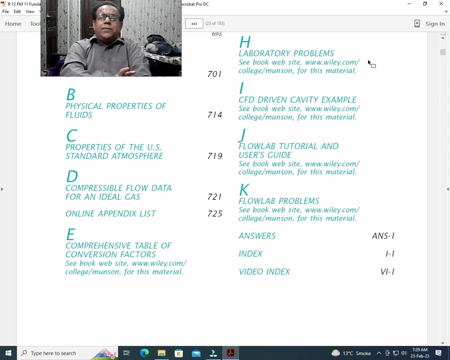 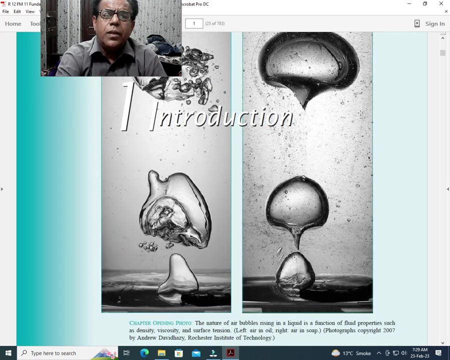 Dynamics, Bernoulli equation, fluid statics, fluid kinematics, finite control volume analysis, differential analysis of fluid flow, viscous flow in pipes, dimensional analysis, similitude and modeling, compressible flow, flow over emerged bodies, open channel flow, turbo machines, and indexes, indexes give, oh no, index page is not given, index page is not given, ok, yes, now we can move to next book consists of 348 pages, 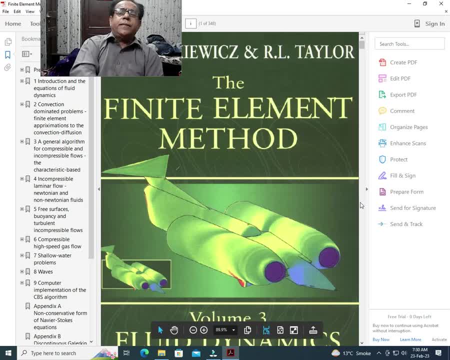 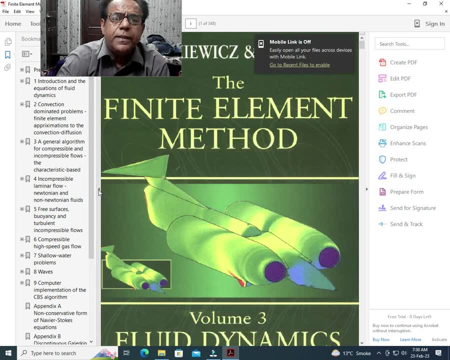 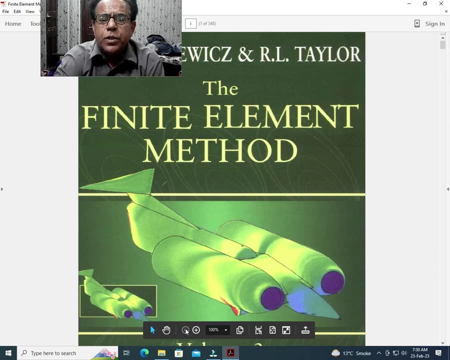 348 pages, 348 pages, this is the book which consists of 348 pages, ok, 348 pages in accordance with soft format arrangement, ok, not hard copy arrangement, ok, this is the situation, ok, this is the situation, this is the situation, 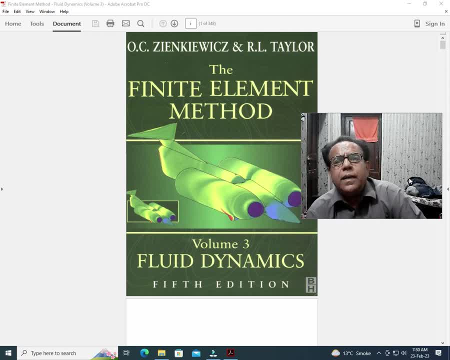 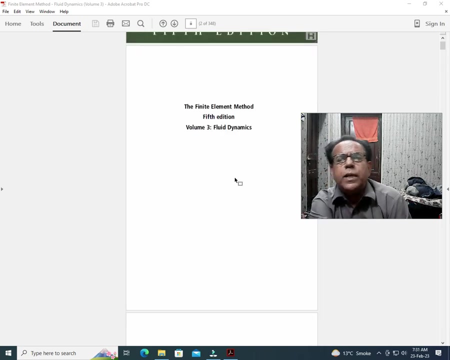 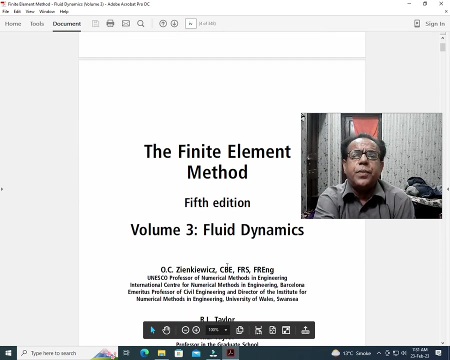 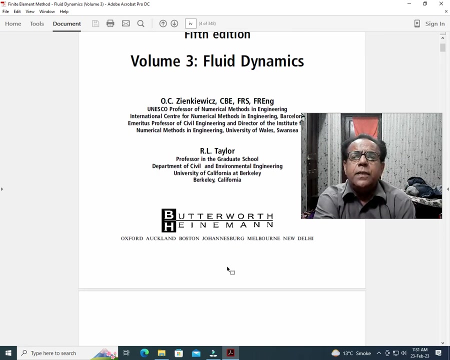 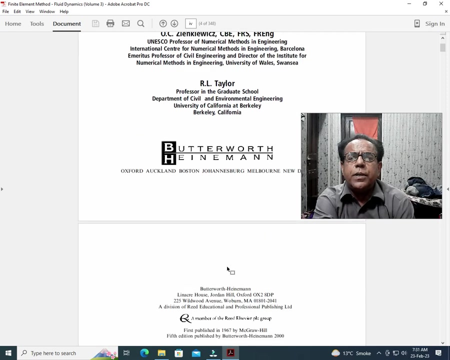 OC Zane Kevicks and R.L. Taylor, ok, the extent of R.L. Taylor, we do not feel any difficulty, but first author seems to be very nutty, ok, OC Zane Kevicks, OC Zane Kevicks, ok, the finite element method, volume 3, fluid mechanics, 5th edition, ok, anyhow, we move forward, the finite element method, 5th edition, volume 3, fluid dynamics, the finite element method, 5th edition, volume 3, fluid dynamics, OC Zane Kevicks, CBEFRS, FR Engineering, R.L. Taylor, ok, Butterworth Honeyman, 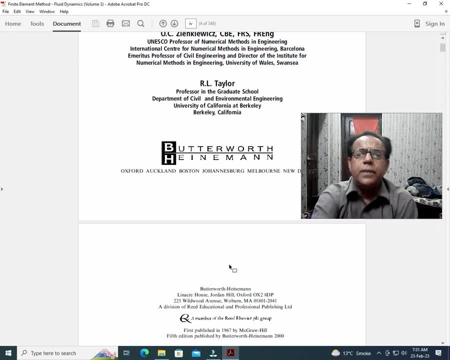 ok, Butterworth Honeyman, ok, Butterworth Honeyman, is the publisher of this book, 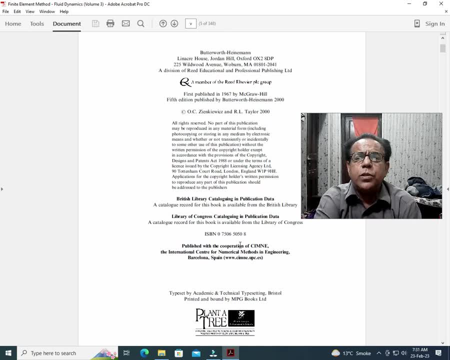 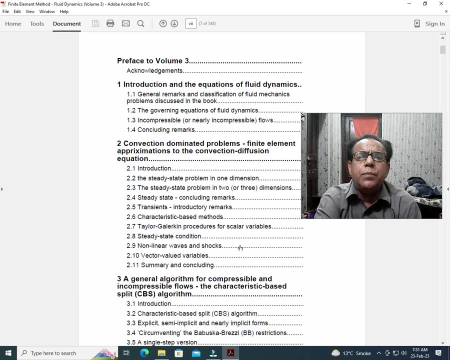 and its year of publication is 2000, ok, 2000, this book was published in the year 2000, and now we come to its contents, 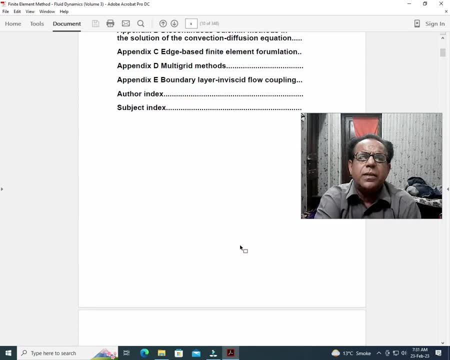 dear students, no need for contents, contents similar, see, all these books have, see, all these books have, 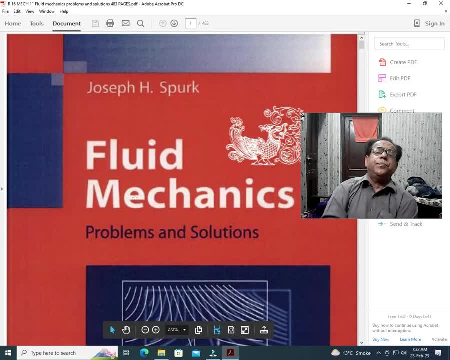 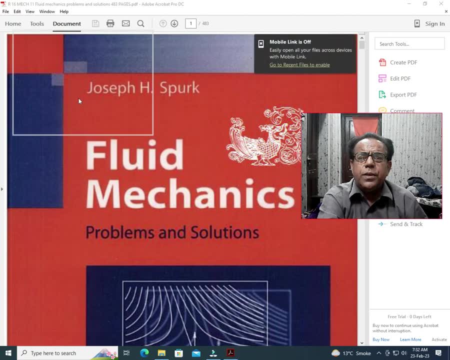 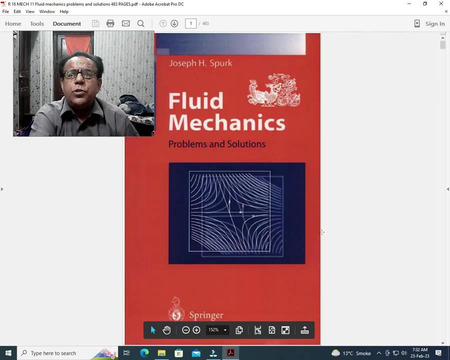 contents is because their title is similar okay here in name is slightly different okay Joseph H is a perk Joseph H spark of fluid mechanics problems and solutions Springer is its publisher Springer is it's a publisher Springer is its publisher 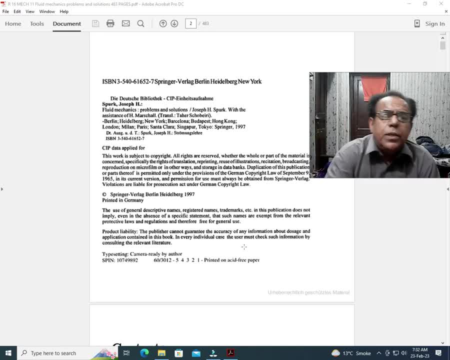 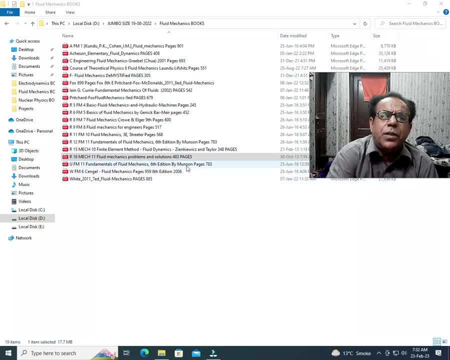 1997 okay this book seems to be seems published in 1997 now contents are noble dear students and offer we have opened an a book books and seen their content say 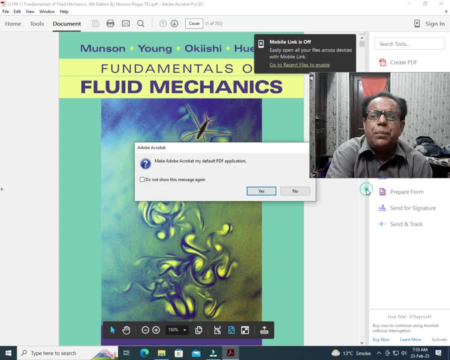 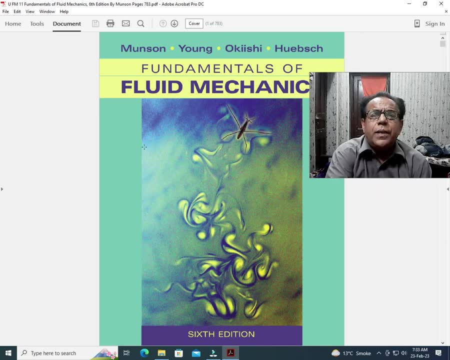 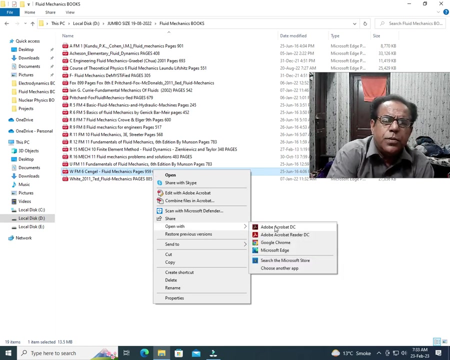 perhaps this book is a overlap are repeated and we have seen this book in our previous book yes I think perhaps this is an overlapping all the most addition may be different however we have this is not a new book this is old book S and X fundamental 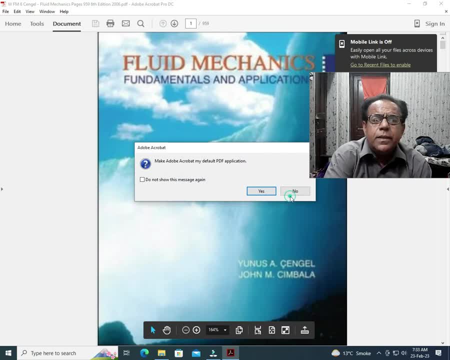 mechanics yes dear students this is the situation here fluid mechanics fundamentals and applications 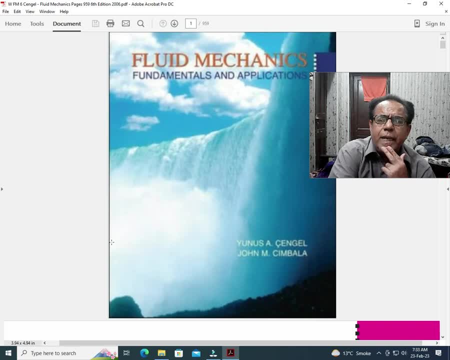 Jonas a single okay Eunice is usually Pakistani Muslim name but here it may be some more in other sense okay why you and us Eunice a C E N G L single Eunice a single and Joe John M Simbala okay 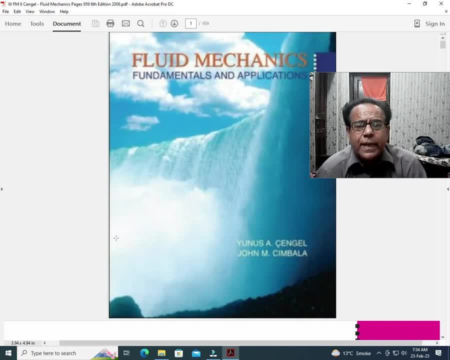 Eunice a single Eunice a single and John M Simbala Eunice a single and John M Simbala okay 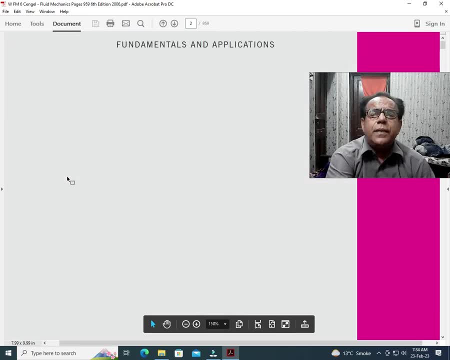 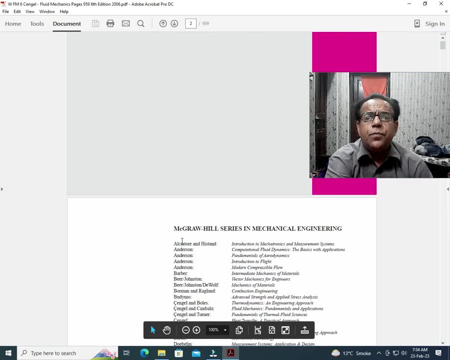 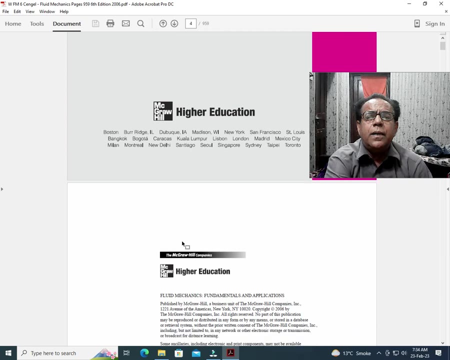 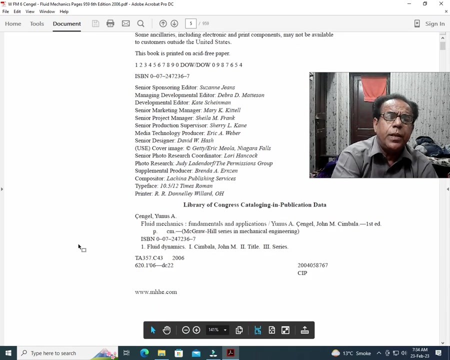 fluid mechanics fundamentals and applications okay okay okay macro hill is its publisher the fluid mechanics fundamentals and applications macro hill higher education now we see it's a year of publication okay year of publication year of publication 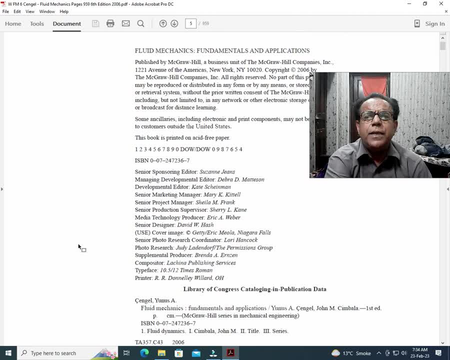 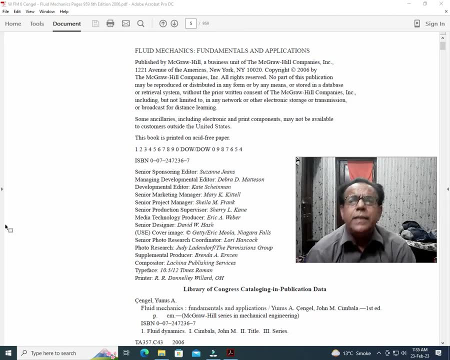 that's probably the fact that here yes your publication is not very important for us but as a formality this 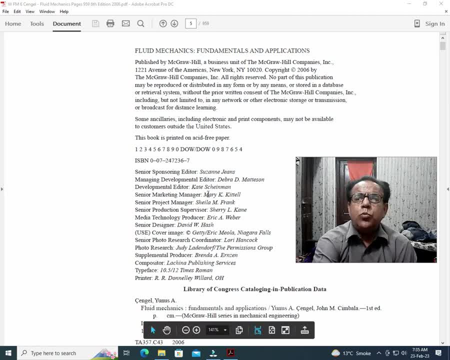 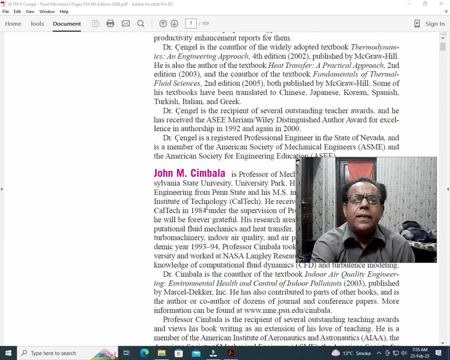 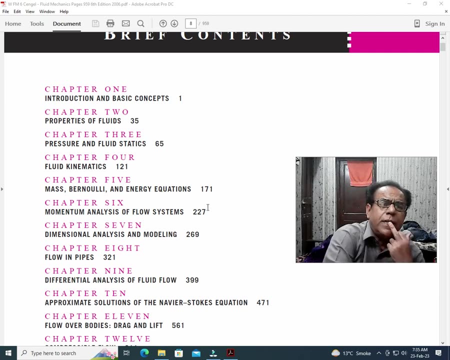 book was published in the year 2006 okay 2006 2006 okay Eunice a single and John a Simbala these are the contents okay introduction and basic concepts of properties of fluids pressure and fluid statics 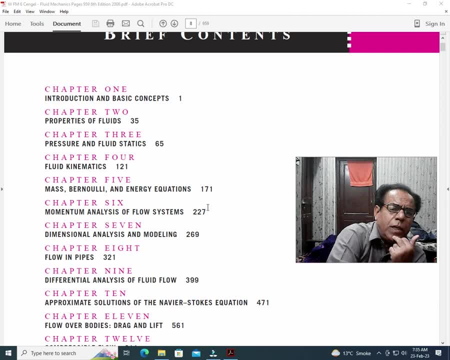 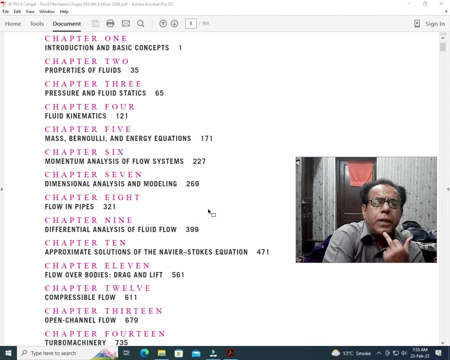 fluid kinematics mass Bernoulli and energy equations momentum momentum analysis and flow momentum analysis of flow systems dimensional analysis and modeling flow in pipes differential 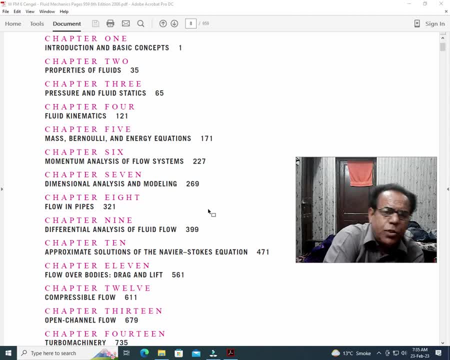 analysis of flow approximate solutions of the Navier stokes equation flow over bodies drag and lift compressible flow opened relations effective at moving etc for Solve gravity of upstream fluids during power generation nutrition total inputашивая お金だからし 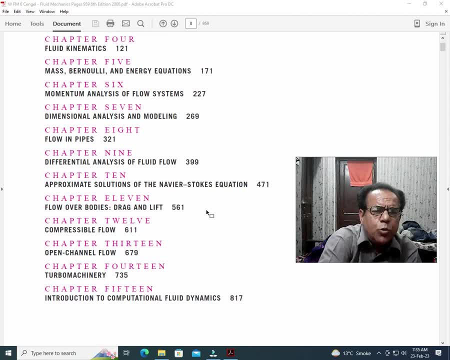 channel flow turbo machinery introduction to computational fluid dynamics anyhow we leave 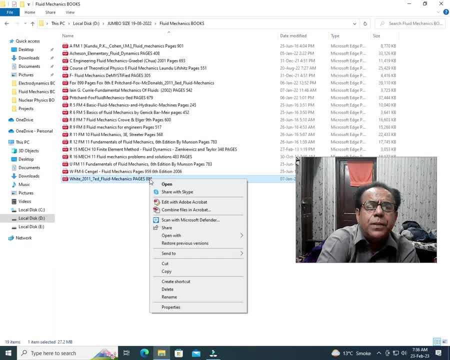 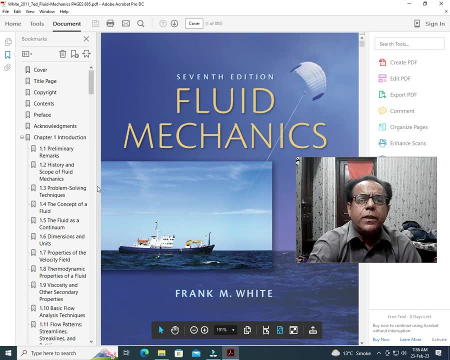 this book and last book consists of 885 pages last book consists of 885 pages this is seventh edition of fluid mechanics okay seven hundred this book is of 885 pages 885 pages 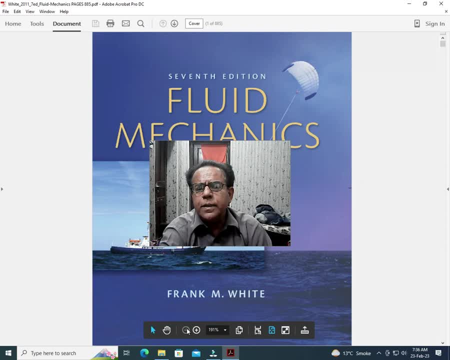 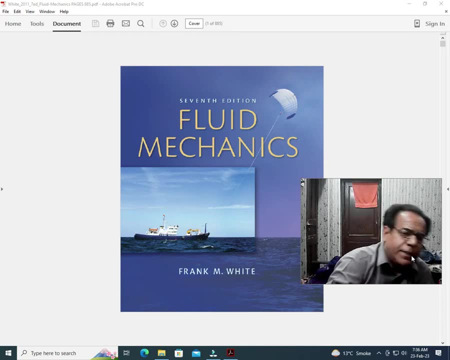 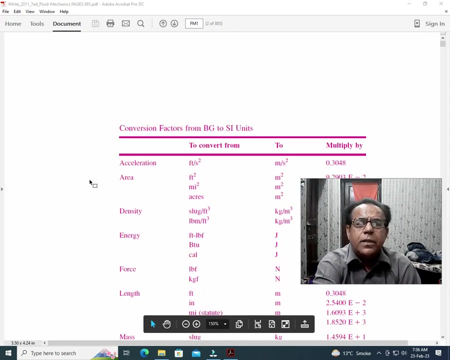 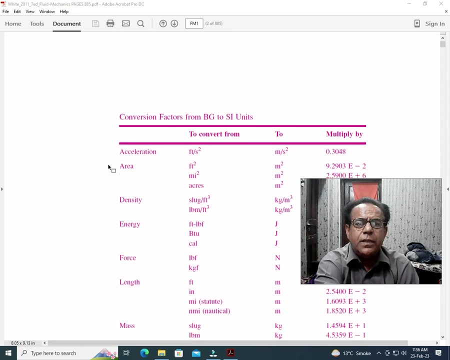 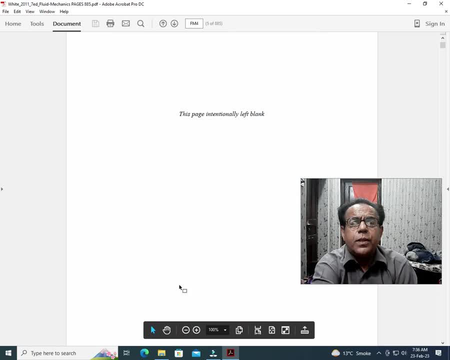 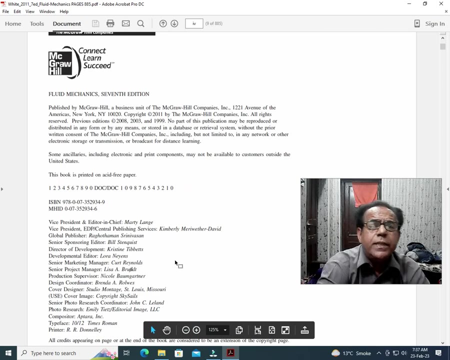 fluid mechanics fluid mechanics seventh edition frank m white frank mackerel is its publisher now we come towards its year of publication okay year of public 2011 okay 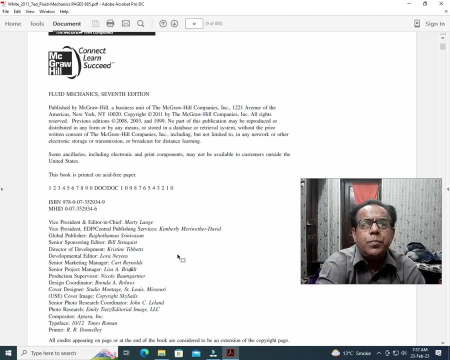 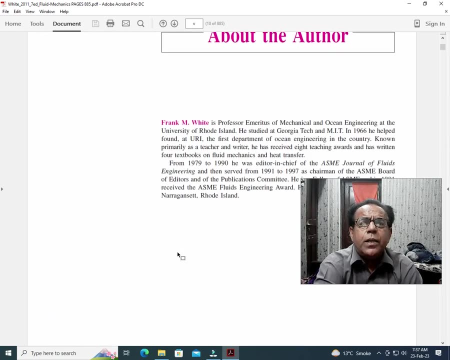 2011 and previous years of publication are 1999 2003 2008 okay in a sense order 1999 2003 2008 and then 2011. now we come towards its contents contents okay introduction 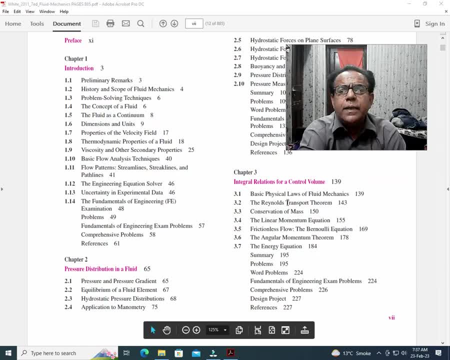 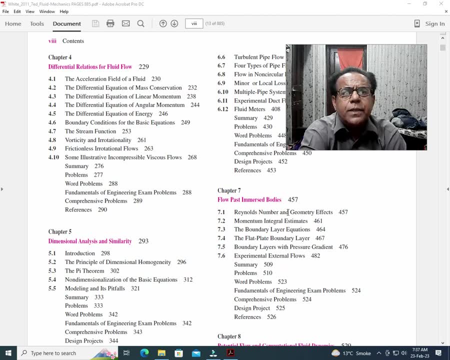 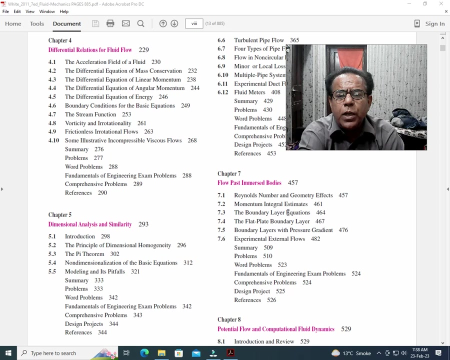 introduction integral relations for a control volume pressure distribution in a fluid differential relations for fluid flow dimensional and similarity not similitude okay anyhow flow past emerged bodies potential flow and 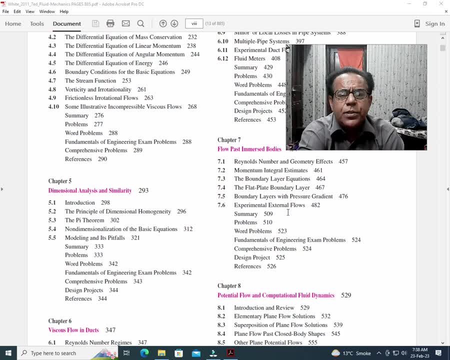 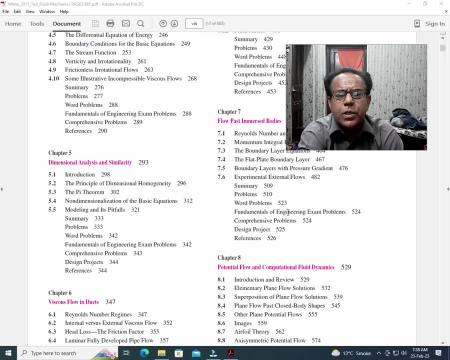 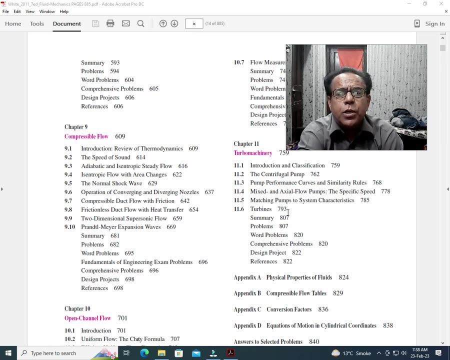 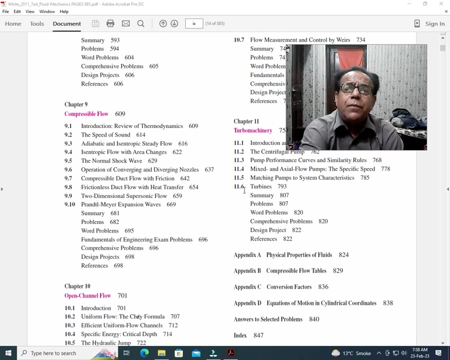 computational fluid dynamics viscous flow inducts partial potential flow and computational fluid dynamics viscous flow inducts potential flow and computational fluid dynamics compressible flow turbo machinery of channel flow and index is given at page number 847 and in our next video we will we will come towards